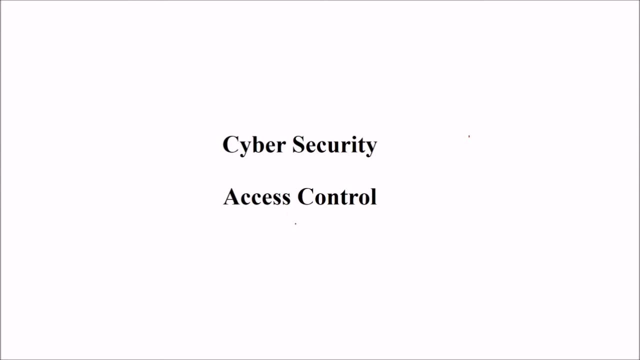 So we are talking about the cyber security In this. we are taking the access control, So we'll see the access control overview, the aspects of access control, that is, identification, the authentication, the authorization and the accountability and the single sign-on. 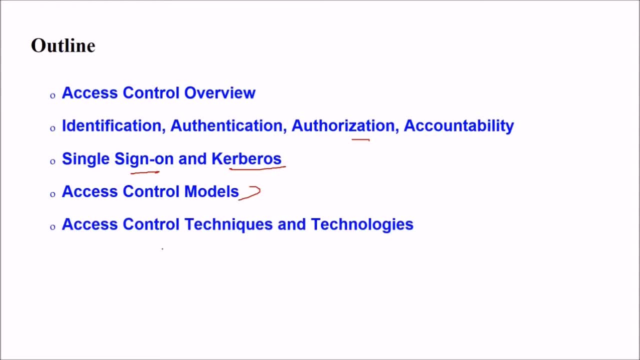 and also the cabros. then the access control models, access control techniques and technologies, and also the access control administration, the monitoring of access control, that is, the intrusion detection and the threats to access control. So what is access control? 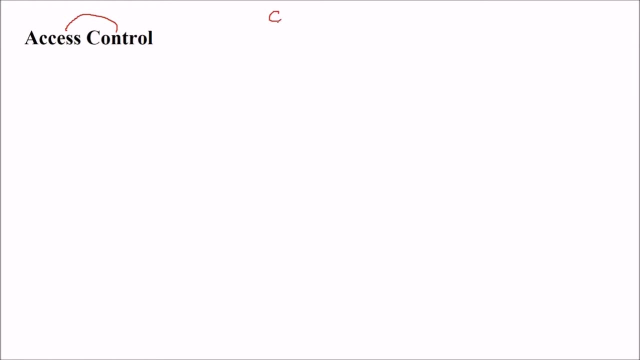 In simple terms, the controlling the access. if, say, someone is there and there are two rooms, Now you want him to enter this room but not the second room, This is a kind of access control. So access control is actually a system which enables you or the authority. 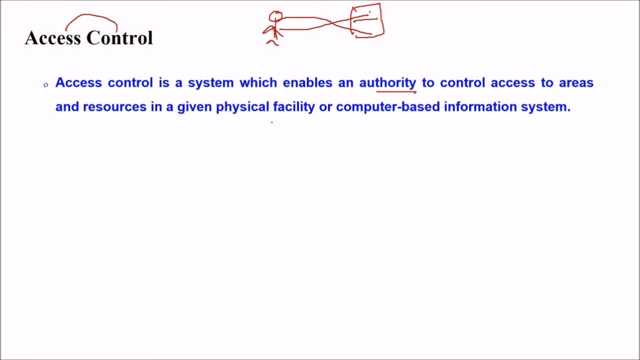 to control access to areas, these areas or resources in a given physical facility or say, a computer-based information system. In this computer-based security, access control includes many things. For example, it includes the authorization of access control, the authentication, it says authorization and also the audit And also it measures the physical. 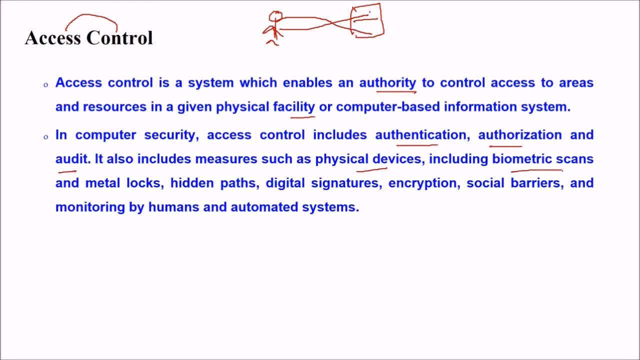 devices. It measures physical devices like the biometric scan- you know your iris and your finger- scans the metal locks, the hidden pass, the digital signatures also, along with the encryption and social barriers, and then also monitoring the humans and the automated systems. 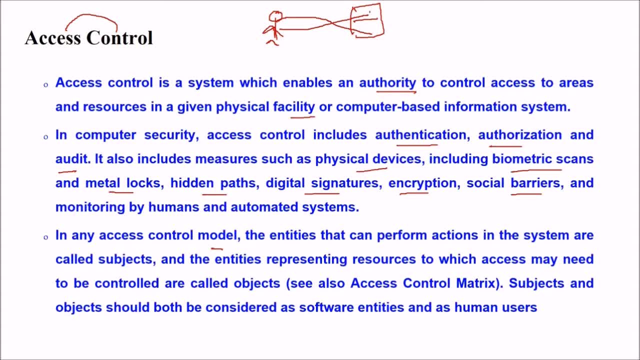 So in access control model, the entities that can perform actions. in the system they are called as subjects. Subjects can perform the actions And these entities, they represent the resources to which access may need to be controlled, And these are called objects. So the subjects: entities that can perform. 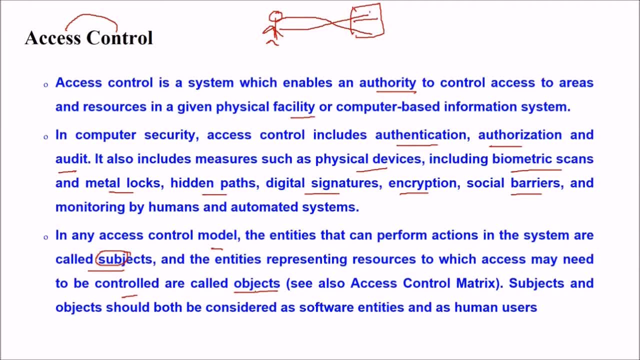 actions in access control model are subjects And objects are what To which access may need to be controlled are objects. We'll also see the access control metrics. So subject and object, these two, subject and object- should both be considered as software entities. 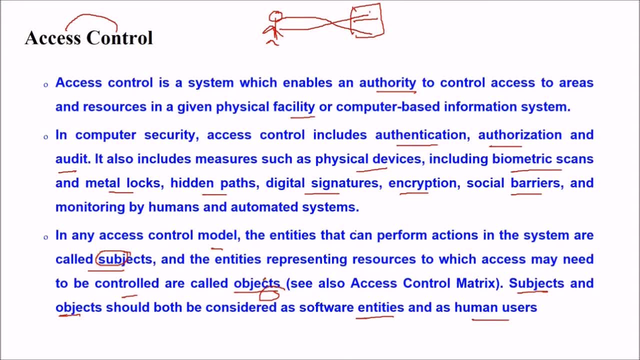 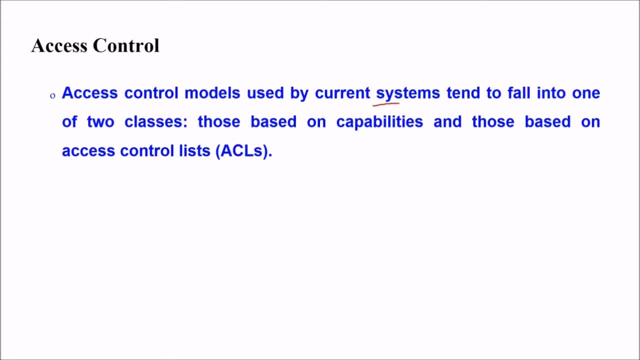 and as human users also. It may be software entities, it may be human users. it may be software entities, it may be human users also. So, access control model used by the present systems. they tend to fall into two classes, two categories, you know. First, 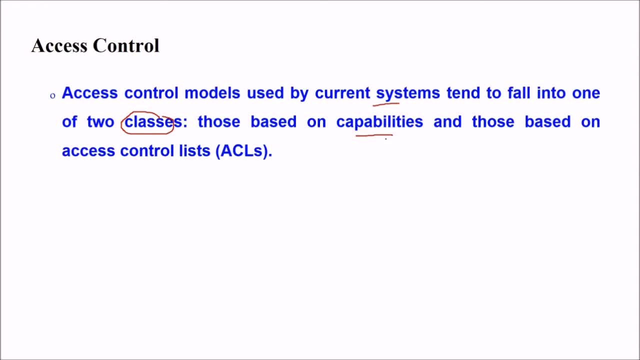 they are based on the capabilities and those which are based on the access control list. So capabilities and access control list, these are the two classes In this capability-based model. holding an unforgeable reference or capability to an object provides an access. 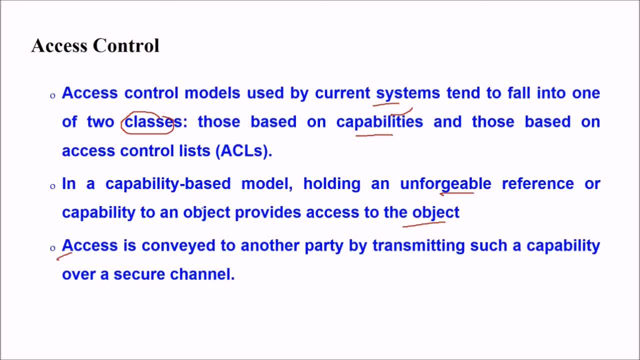 to the object- this capability-based model- And the access is conveyed through the access to another party by transmitting such a capability over certain secure channel. So access is conveyed over certain secure channel, But in the access control list model, the subjects: access to an object. subject: access to an object depends on whether its identity on 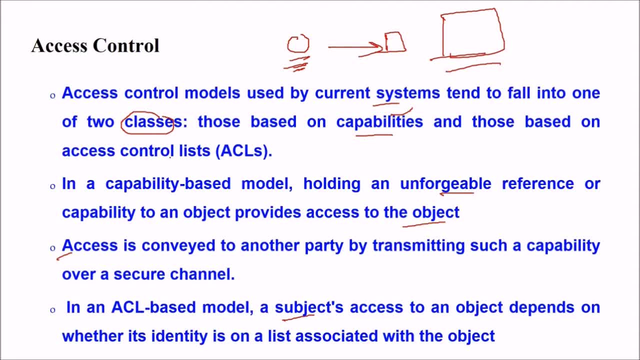 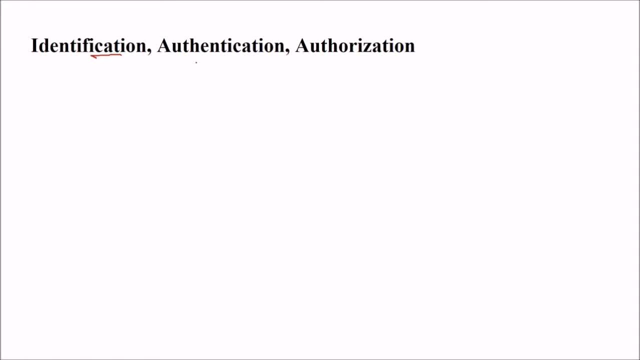 the list, that is, the access control list, is either associated or not associated with the object. Then when we come to the measures of access control, it can be identification, authentication and authorization. The access control system provides the essential services of identification, authentication, authorization and accountability. If you want to control, 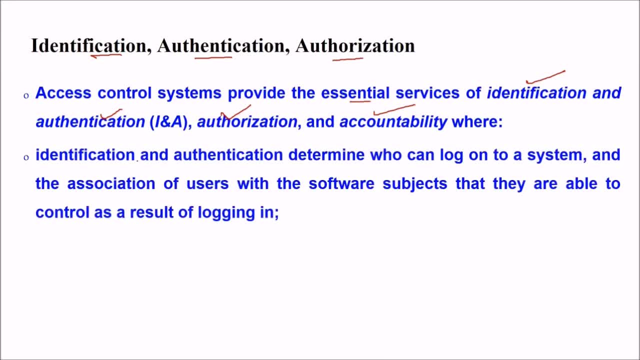 the access, these are the measures, these are the methods, The identification and authentication. here it determines who can log on to the system and the association of users with the subjects they are able to control as a result of logging in, Once they are logged in, which? 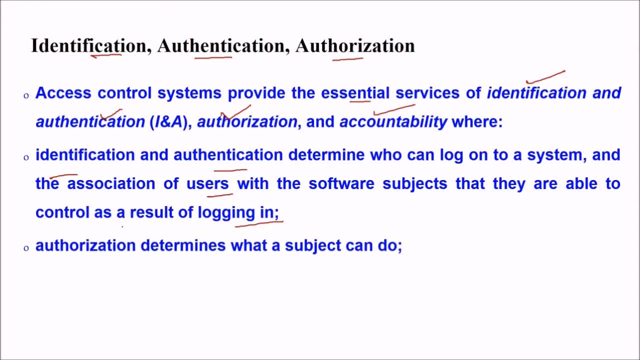 or where they end up in the system by logging in. the system comes in where and to whom they have control. see the authorization determines what a subject can do, what is the possibility, what he is authorized to, and accountability identifies what a subject did. means when he is identified and authenticated, then he is authorized. then after he has done. 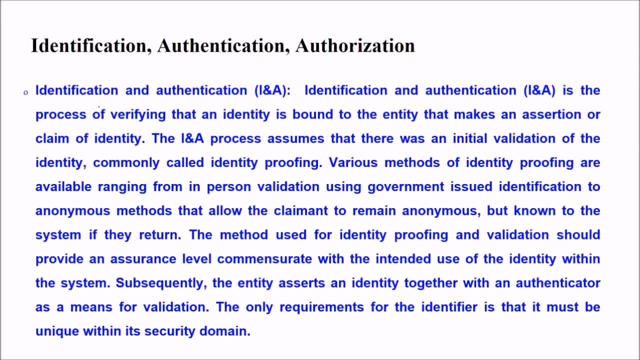 something. the accountability should be there. so, identification and authentication, let us see these two terms. the, these two terms i and a we call it, is the process of verifying that an identity is bound to the identity. that's that makes an assertional claim of identity. if somebody 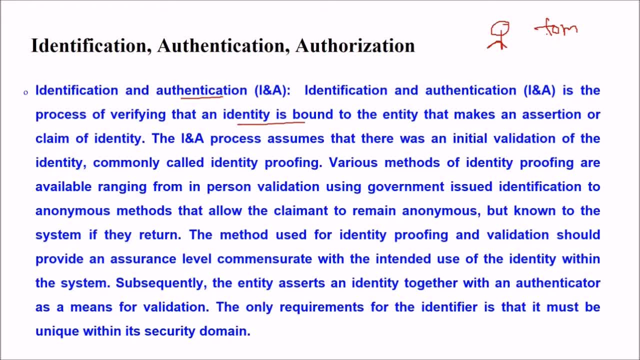 comes and he says: i am tom. whether he is tom or not, no, he can be anybody. so whether he is tom or not, this is the identification authentication. so what is the ia process? it assumes that there was an initial validation of the identity and we can call it as identity proofing, so certain. 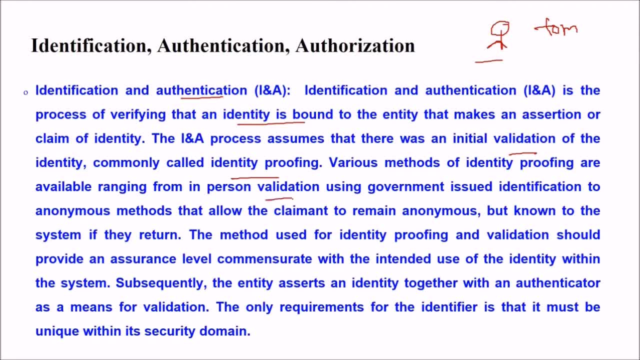 methods of identity proofing are available, right from the personal validation. he may have a government card, identification card to any. you know there are various methods. we can allow the claimant to remain anonymous, but no to the system if, if they can provide the access or they can authenticate, so the method. 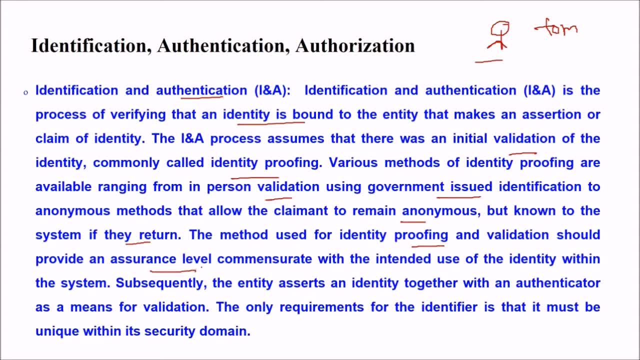 used for identity proofing and validation. they should provide assurance level commensurate with the intended use of identity within the system. so thereby the entity asserts an identity together, together with an authenticator, as a means of validation. so there are two things need to know and the authentication. so together these two, then only we can validate it. so the only requirement 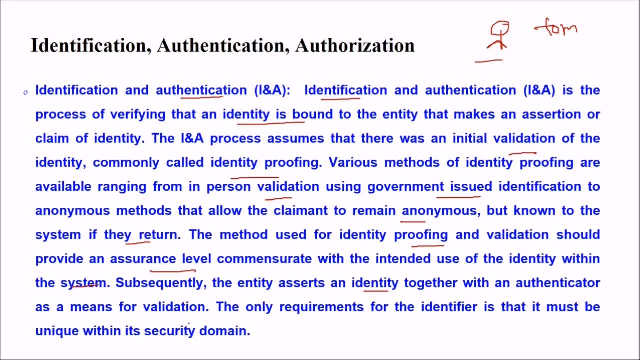 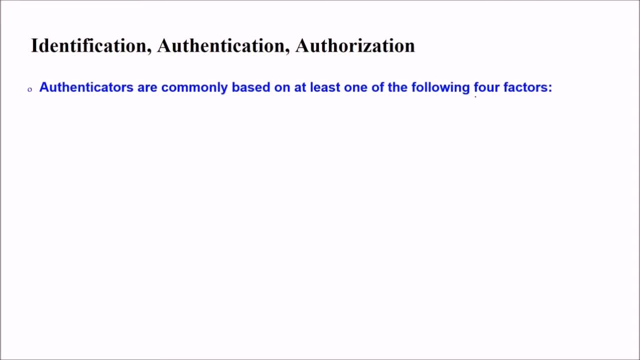 for the identifier is that it must be unique within the security domain. there should not be any chance of ambiguity at all. so authenticators are commonly based on uh. we have four factors, or at least one of the following factors. authenticators are these: first, is something you know, like a, like a pin, personal identification number or a password which is known to you only. 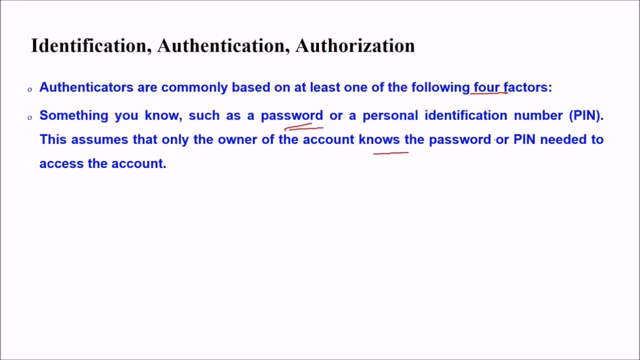 so this assumes that only the owner know, knows, the password or pin of the account. he needed to access the account. then the second is something you may have, only say a physical entity, like a, like a smart card or a security token. so these security token and smart card, 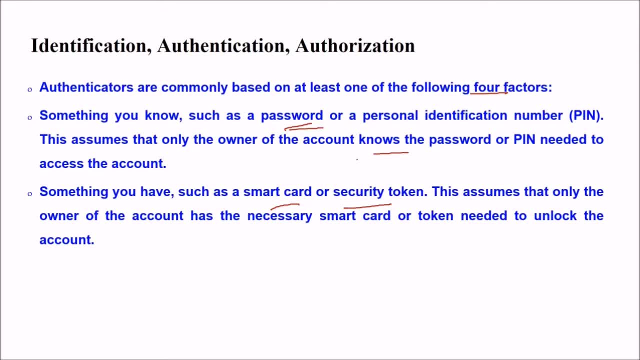 we assume that that can be held only by the person who is, who is actually what he is, you know, trying to tell us that, okay, i am this guy. so this assumes that only the owner of the account has a necessary smart card and token needed to unlock the account, something like. 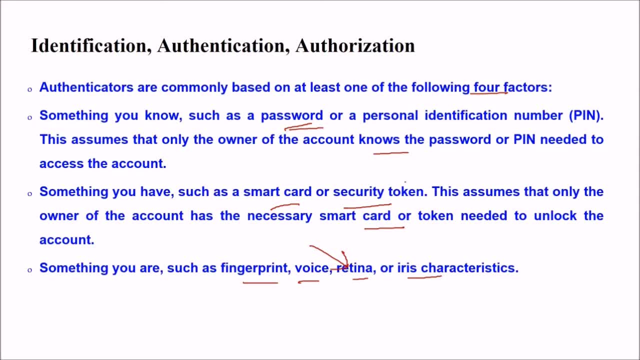 fingerprint, voice, retina and iris. these are the biometrics. so biometrics can only, can only belong to the individual who is trying to access or trying to ask for the authentication and where you are for this, where you are, for example, inside or outside a company firewall or proximity of 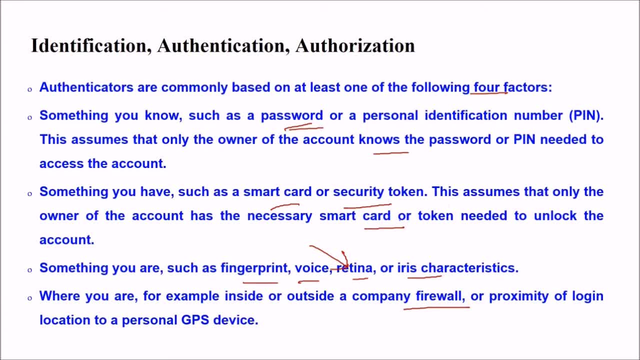 login location to a personal gps device. okay, if you are nearby there to a personal, you can have a personal gps device and you are bound to you know be authenticated. then only the authenticators. you can have a personal gps device and you are bound to you know the authenticators, then only. 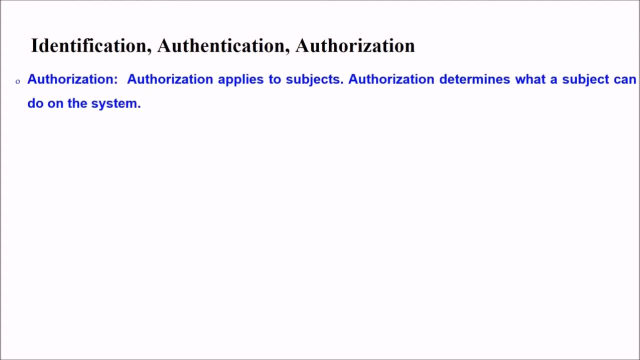 can be invoked, the authorization once the identification authentication subject is complete. then we talk about the authorization only after this. so authorization applies to subjects, to subjects. so authorization tells us what a subject can do on the system. now, for four factors we have seen: by any of these means we can authenticate. but now, when he has come in, what he can do most. 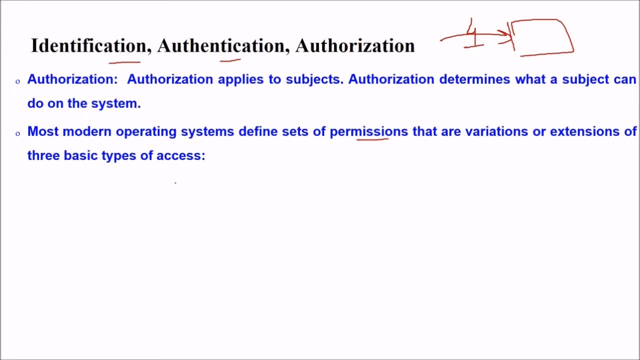 modern operating system. they define a set of permission that a variation or extension of three basic types of access. so let us see. first is read: the subject can only read file contents, list directory contents. he may write. that means a subject can change the content of the file directory which say add: 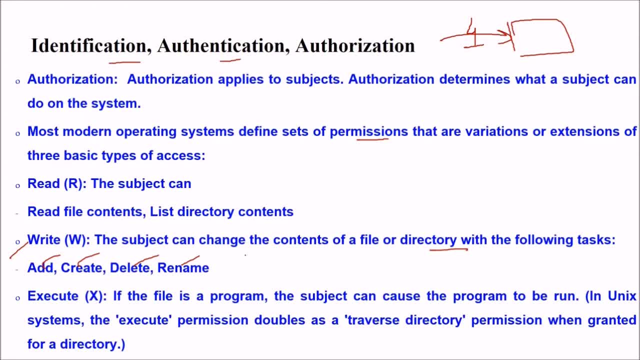 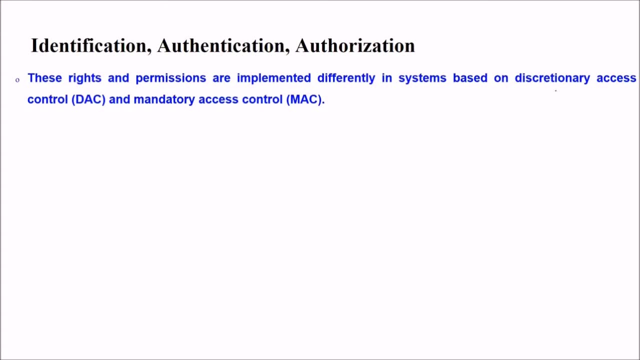 create, delete and rename. he can also execute if the file is a program subject, can cause the program to run. for example, in unix the execute permission doubles as a traverse directory permission when granted for a directory. so these rights and permission, they are implemented differently in system-based on the 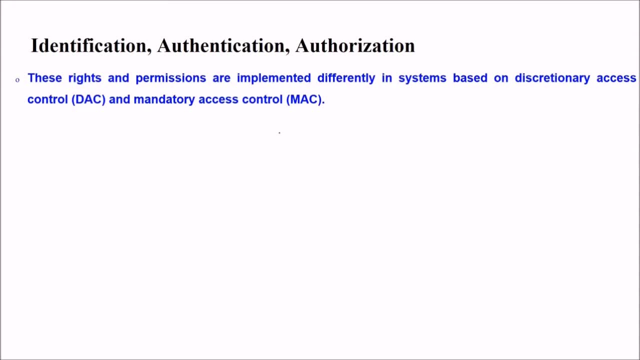 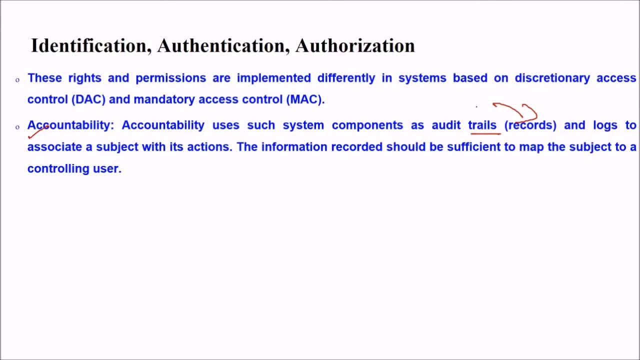 authenticated once he's authorized. now for this, this, this objects. now you need to have auditors. that is, record and locks to the associate a subject with their section, so the information recorded should be sufficient enough to matter. map this subject to a controlling user, these audit trails for a contability. 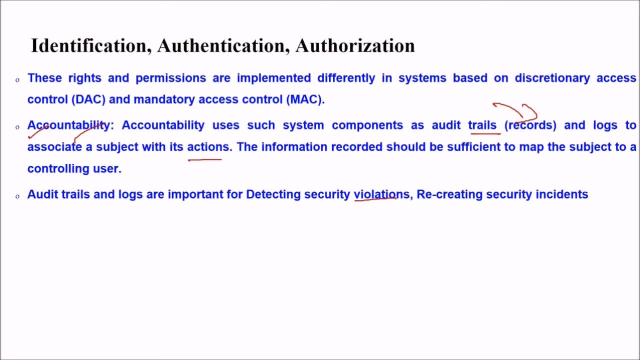 and the logs are important for detecting security violation and recreating if certain incident has happened. security lapse has happened. so if no one is regularly viewing your logs and they are not maintaining, or they are not maintaining, a secure and consistent manner, they may not be admissible. 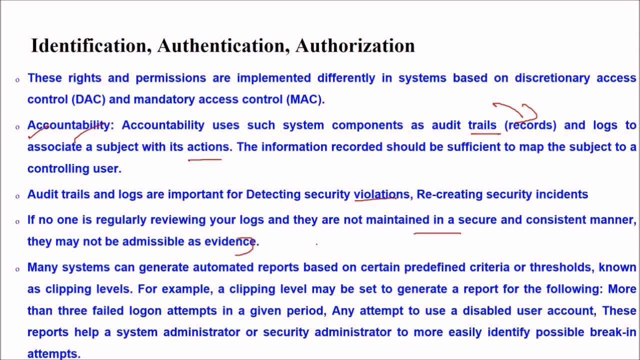 as evidence right. many systems can generate automated reports. there is no certain predefined criteria or thresholds like clipping levels, just for example, a clipping level may be said to generate a report for the fall if you have more than three failed logger attempt. somebody is trying to attempt login and he failed for three times, he failed thrice. or say, say you know any. 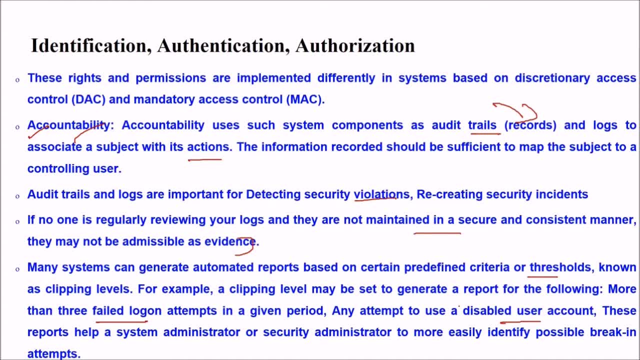 attempt to use a disabled user account. so this, these reports help a system administrator to, or the security administrator per se to more easily identify the possible break-in attempts? not, no, it is not possible to to find out and to to monitor each and every login and the activity. 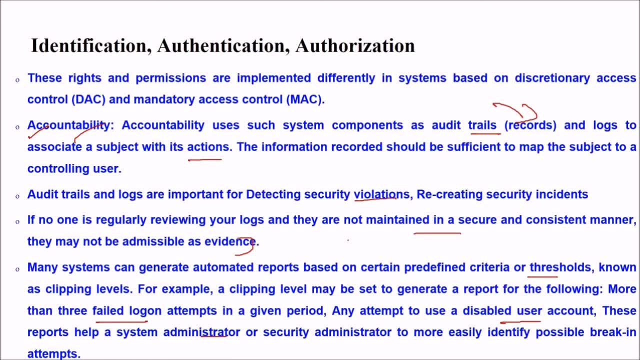 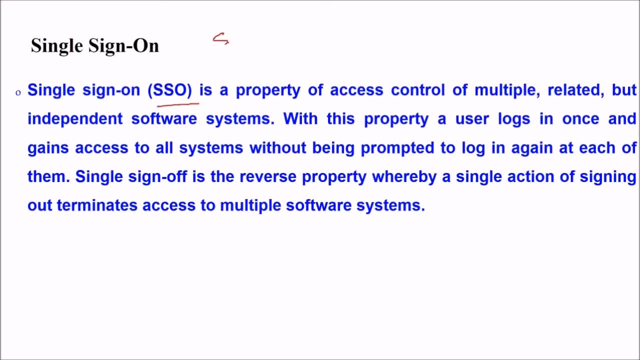 but but the spurious or these suspicious activities can be can be seen. what is signal sign on? sso? signal sign on? this is a property of access control for multiple related but independent software system. multiple related but independent software system, for example in google. what you do? 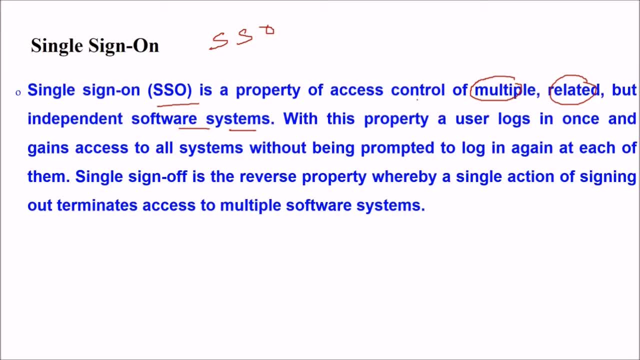 you have a gmail account, you log on to gmail. you are logged on to youtube. you are logged on to gmail. you are logged on to google plus. so, with this property of access control, you are logged on to use a log only once and then of that system, without being prompted to log in again at each. 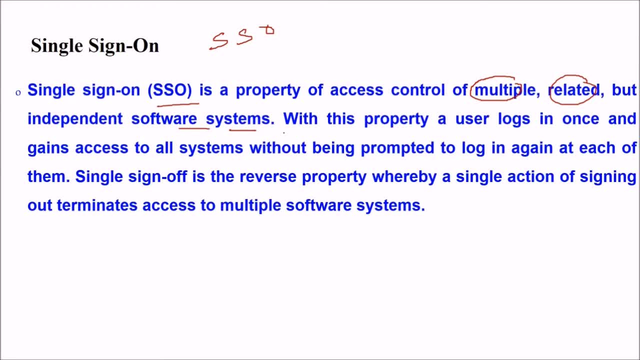 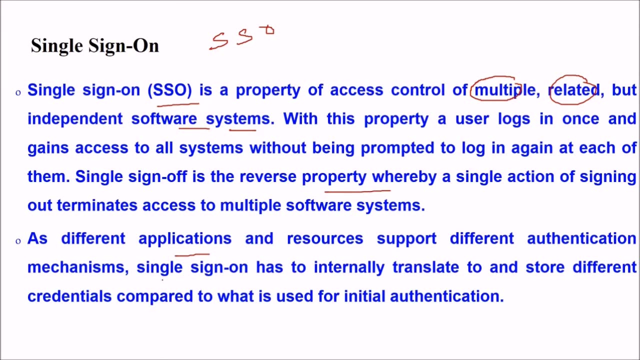 each of them. there are multiple software system, but they are, they should be related. so single sign off is the reverse property whereby a single act of action of signing out terminates access to multiple software system. so as different application and resources, they support different authentication mechanism. the single sign on has to internally translate and store different 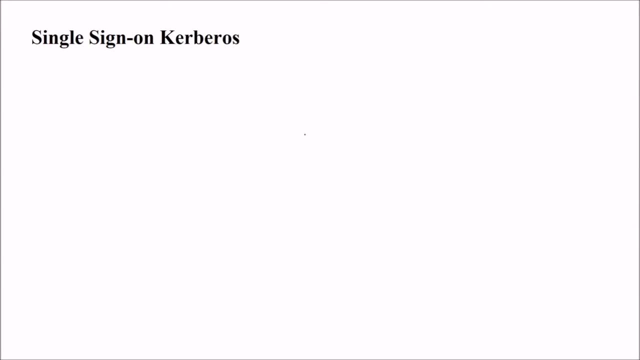 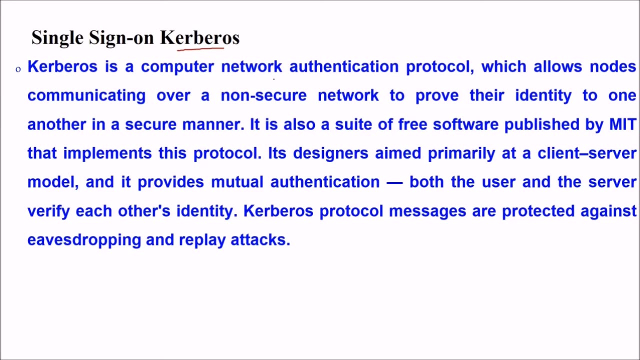 credentials compared to what is used for initial authentication. Then we talk about the Calgros single sign-on. Calgros, So Calgros is a computer network authentication protocol which allows the nodes, over a non-secure network, to prove their identity to another- one another- in a secure manner. So it also suits a free software. 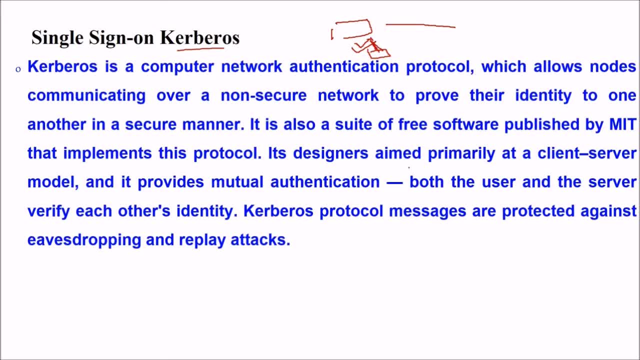 published by this MIT that implements this protocol. So the designer aimed primarily at a client server model. So it provides a mutual authentication, but the user and the server verify each other's identity. This Calgros protocol messages. they are protected against the eavesdropping also and replay attacks. So if you are Calgros, signed on or verified. 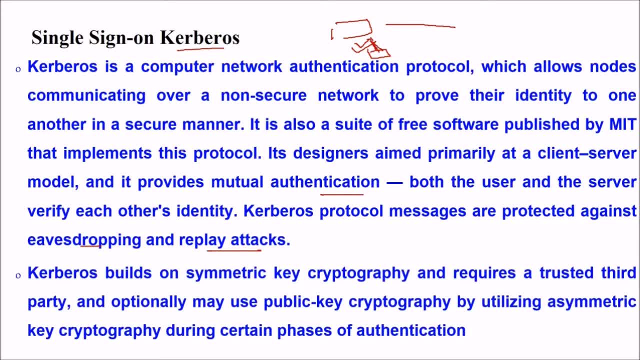 you may assume that you are away from eavesdropping and replay attacks. So what Calgros do? it builds on a symmetric key cryptography. It is built on. Calgros is built on a symmetric key cryptography and it requires a trusted third party. It requires a third party and actually may. 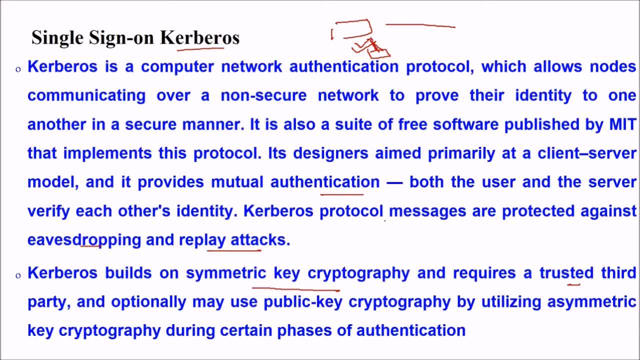 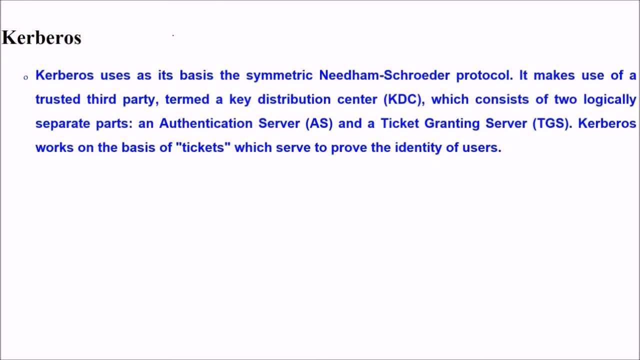 use public key cryptography by utilizing the asymmetric key cryptography during certain phase of authentication. So Calgros uses as its basis the symmetric Needham Schroeder protocol. We will call it as NS protocol. So it makes use of a trusted third party. We know it as. 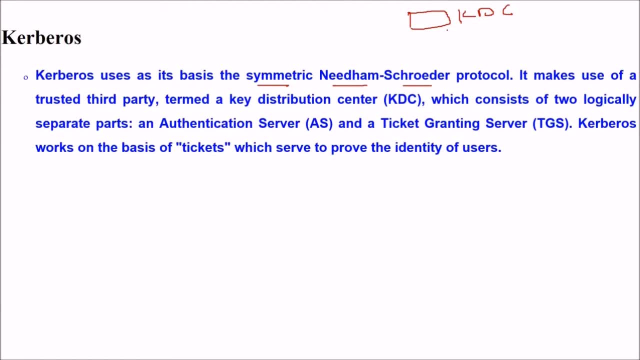 key distribution center which consists of two logically separate power: It has AS authentication servers and the other is ticket granting servers, TGS. So Calgros works on the basis of tickets itself to prove the identity of the users. So if you are a user, you will go to this server and 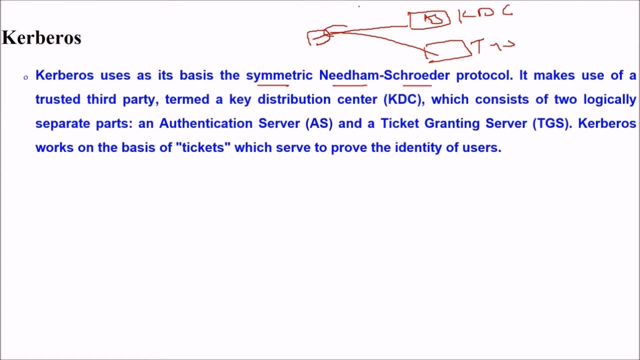 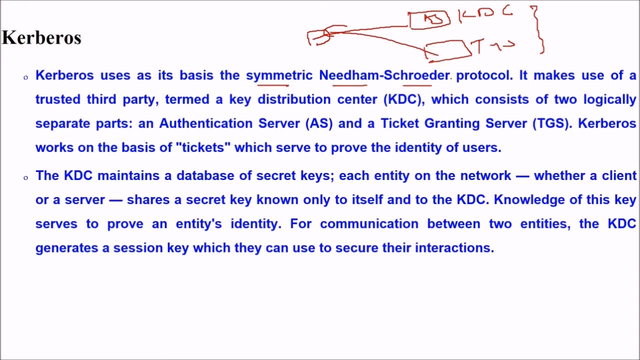 this TGS ticket granting server will give you their ticket granting ticket. So this KDC maintains a database of securities. each entity on the network, whether a client or a server, So they share their shares. a secret key known only to itself and to the KDC. So knowledge of this key proves or serves. 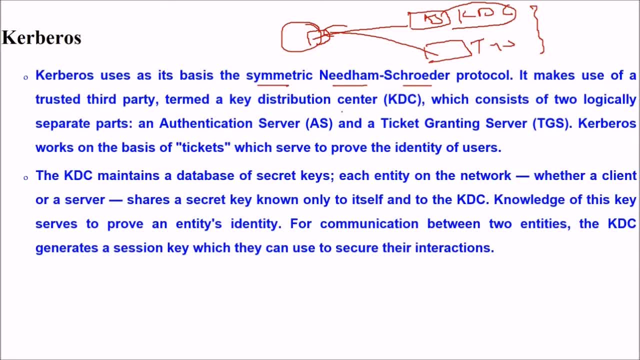 to prove the entity's identity? And what about the communication between two entities? The KDC generate a session key which they can use to secure their interactions or communication. So the security of the protocol relies heavily on the participants which are maintaining loosely a synchronized time. 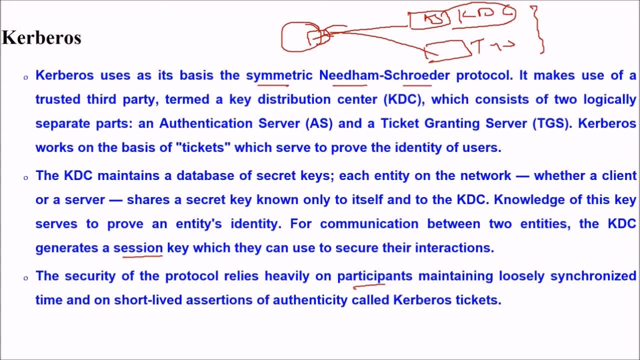 and on a very short-lived assertion of authenticity, which are known as Calgros ticket or ticket granting ticket. Calgros is a very well-known company which is known as Calgros ticket or ticket granting ticket. Calgros is a very well-known company which is known as Calgros ticket or ticket granting ticket. 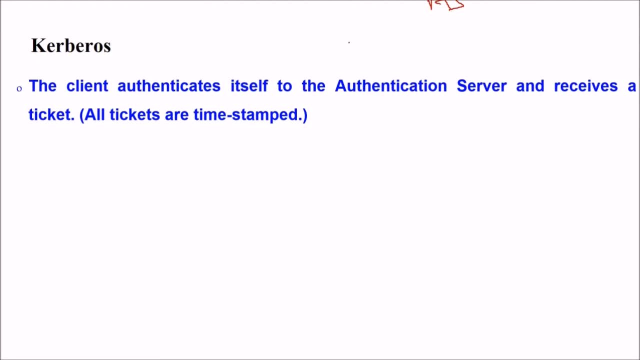 The client authenticates itself to the AS and receives a ticket- TGT ticket- granting ticket- from the Calgros AS. So all tickets are time stamped, that is for session. So it then contacts the ticket granting server, TGS, and uses this ticket to demonstrate as identity. now TGT. 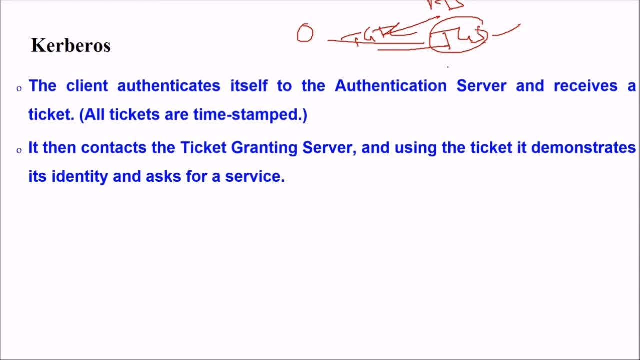 And using this ticket it demonstrate its identity and ask for a service to TGS. So if the client is eligible for the service, then the ticket granting server- TGS server- sends another ticket to the client. Now again, one more ticket is sent to the client. 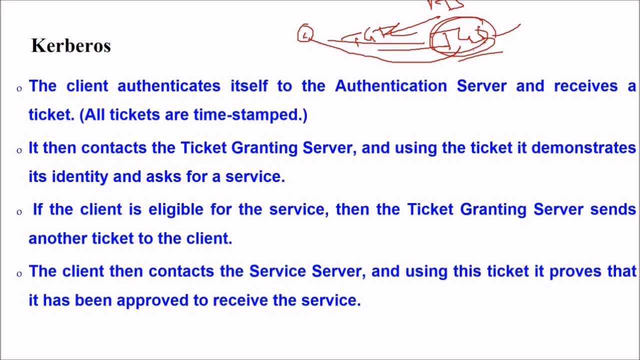 Now again, one more ticket is sent to the client. Then this client contacts the service server. Now you have a server. so these two action has to be taken so that the access to the server can be ascertained, and using this ticket, which is provided by the ticket granting servers this TGT. 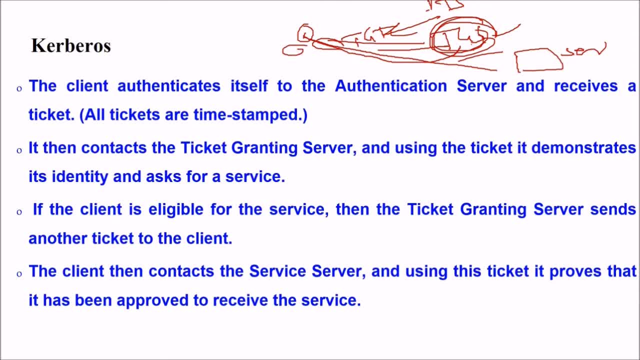 after TGT, TGS has provided another ticket. So using this ticket, the ticket granting server- the client contacts the service which is provided by the server and, using this ticket, it proves that it has been approved to receive the service from the this authentication server and ticket granting. 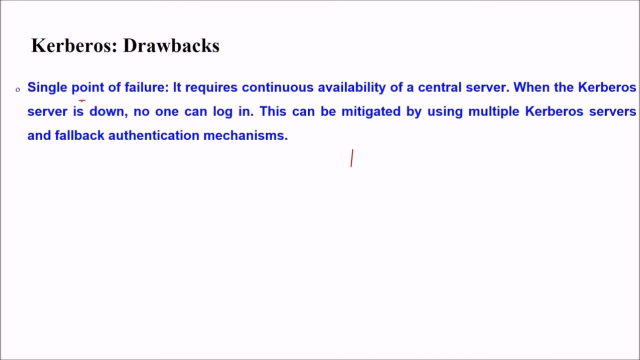 server. But there are drawbacks of Calgros. that is single point of failure. You need to have a continuous availability of the central server, that is, AS and TGS. So when the Calgros server is down, no one can log on. How can you log on? because you don't have that ticket which is provided by 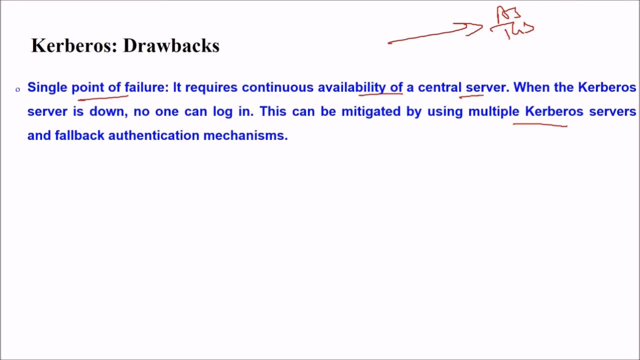 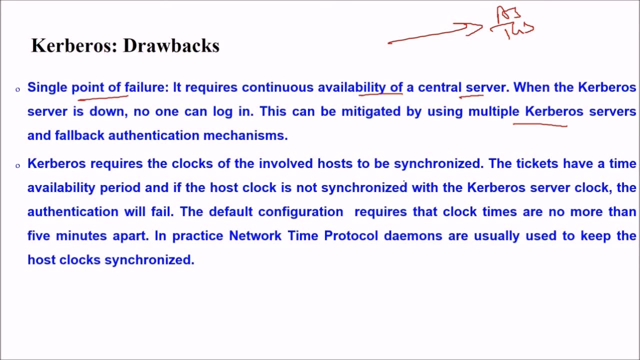 the token actually provided by TGS. So this can be mitigated using the multiple Calgros server and you can also have a fallback authentication mechanism. And this Calgros requires the clocks of the involved host to be synchronized- that because the the tokens are time stamped. 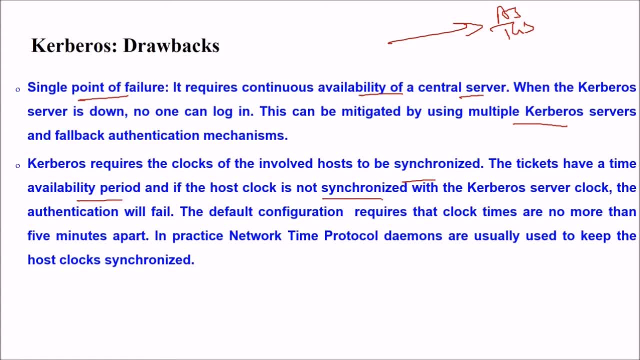 The tickets have a time availability period and if the host clock is, they are not synchronized in the Calgros server clock. the authentication is bound to fail. So the default configuration requires the clock times or they are no more than five minutes apart. But in practice the network 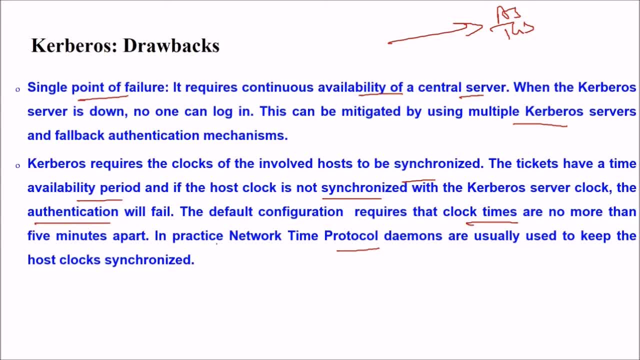 time protocol, daemons are usually used to keep the host called synchronized And the administration protocol, this is. this is not standardized and differs between the server implementation. also, And since all the authentication is controlled by KDC, only you know these two KDC, this compromise. 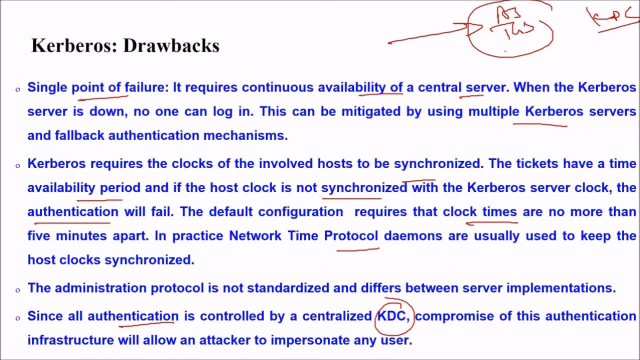 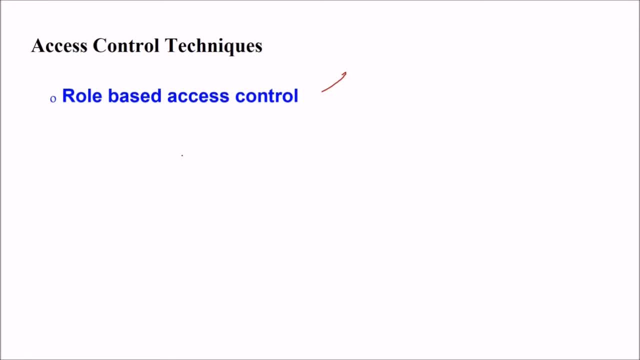 of this authentication infrastructure will allow a attacker actually to impersonate any user. So KDC is important. So access control we were talking about. what are the techniques? It can be role based access control. It can be constrained. user interfaces: It can be. access control can be based. 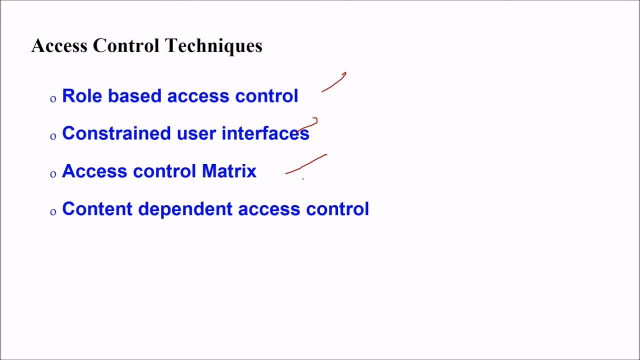 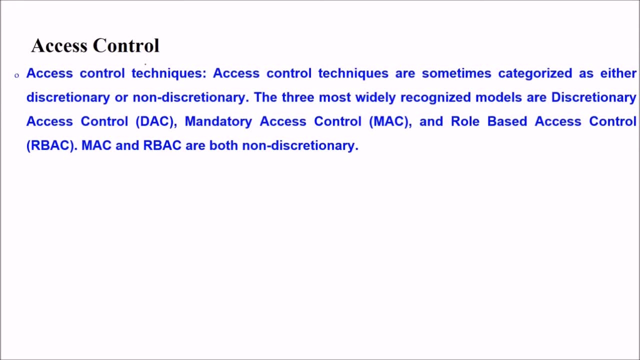 on access control metrics It is. it can be based on content dependent access control or content dependent access control. these two are simultaneously. So access control. how is access control first technique, access control technique, So access control technique, are sometimes categorized as either the discretionary or non-discretionary. So discretion is important. So the three most widely: 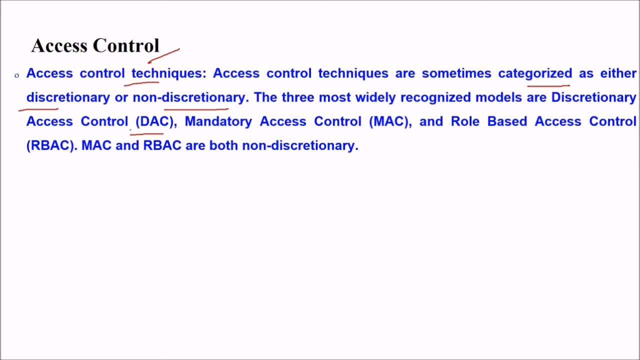 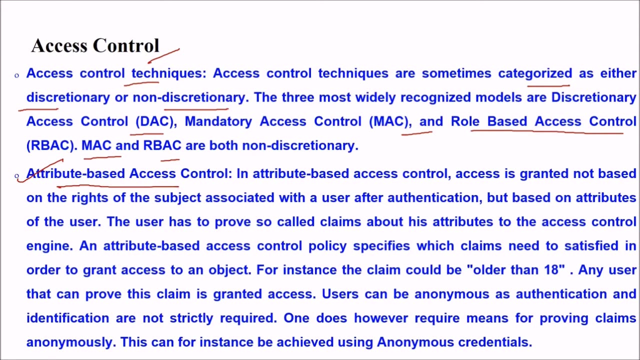 recognized models. they are: DAC, discretionary access control. MAC, that is mandatory access control. the RBAC, that is role based access control. So this MAC and RBAC, both are non-discretionary. The in Debate através access controlакtitibut based access control: the access is granted, not based on the right of the subject associated with the. 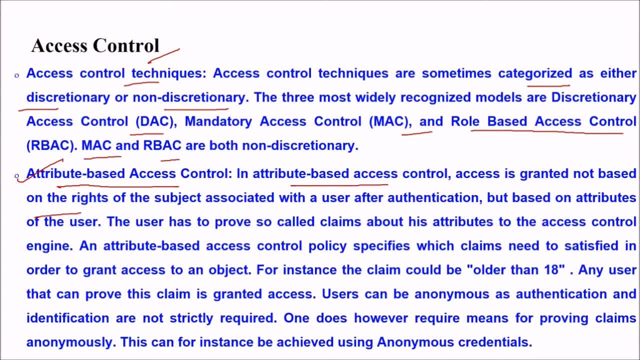 user after it application. But it is based on the attribute of the user, Atribute of the user. It is based on the attribute of the user. So user has to prove, so called claim, that his attribute to the control, to control access engine. He has to prove its claim to the control engine. So this attitude. based control, access control policy. it specify that claims to control to the key controls, that access control ingent. So it is data based control. so illustrations like this, which is to be 여� 8 00 Hospital, You have an presentation and any acti. 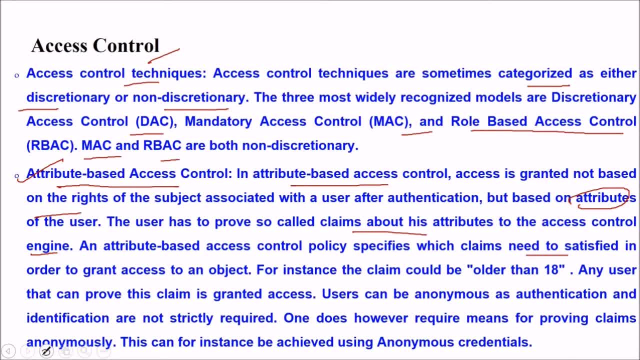 decisions that you want to get Ace earlier. Ajfer, have three ve бывает bets a suppository points on how to use control If I have a volunteer, a registered TH post for the control task, so that you are like me, dont generate an claims need to satisfy in order to grant access to a subject. Let us give an example. Just assume, 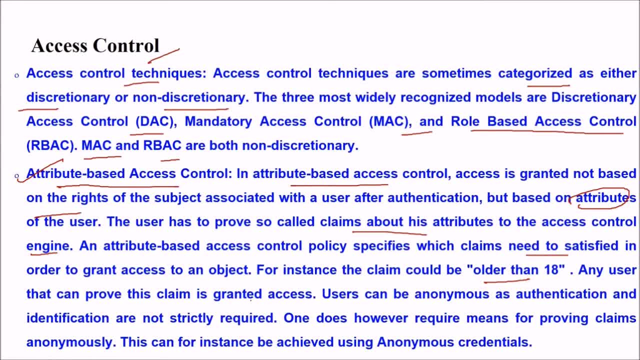 that the claim is older than 18.. So any user that can prove his claim is granted access. He is more than 18 years of age. So users can be anonymous, as authentication and identification are not strictly provided And one does have a required means for providing claims anonymously, This can: 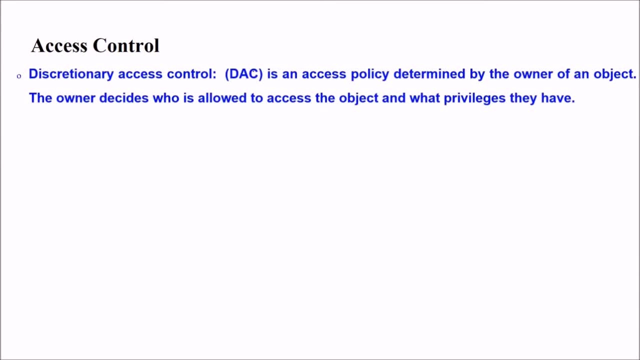 for instance, be achieved using the anonymous credentials. What about DAC? Discretionary Access Control? DAC is an access policy which is determined by the owner of the subject- owner of the subject. So the owner decides who is allowed to access the object and who privileges. 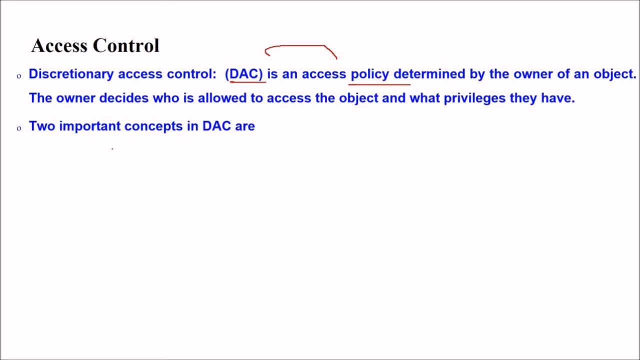 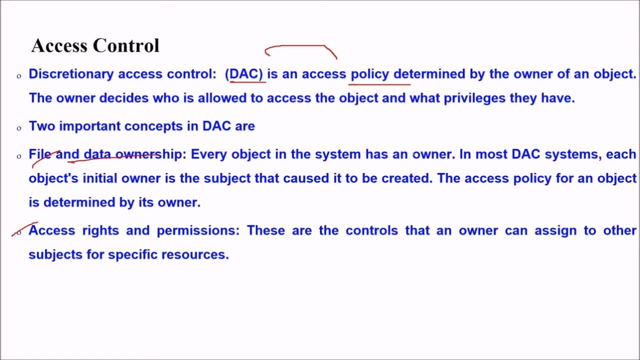 what privileges, what possibilities he may have. So there are two important concepts of DAC. First is file and data ownership, then access, write and permission. File and data ownership means every object in the system has an owner And in most DAC system each object's initial. 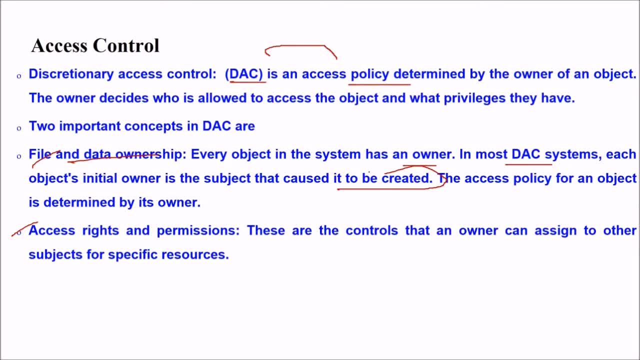 owner is the subject that caused it to be created. So the access policy for an object is actually determined by the owner who has created. What about the access write and permission in the DAC? that is discretionary access. Now let's have a look at the third and final concept, which is the owner and access control. 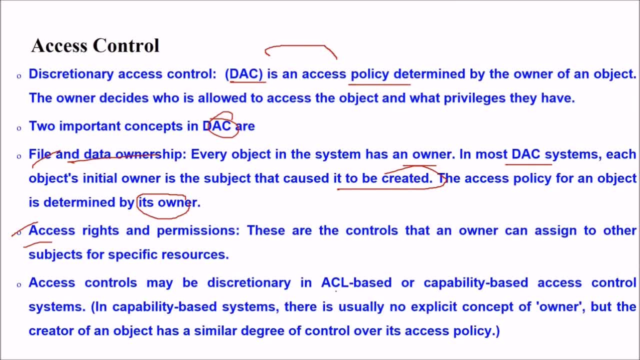 These are the controls that an owner has imposed or he can assign to the subjects for certain specific resources. The access control may be discretionary in ACL based and capability based access control system. In capability access based access control, there is usually no explicit concept of owner at all, But the creator of the object has similar degree of 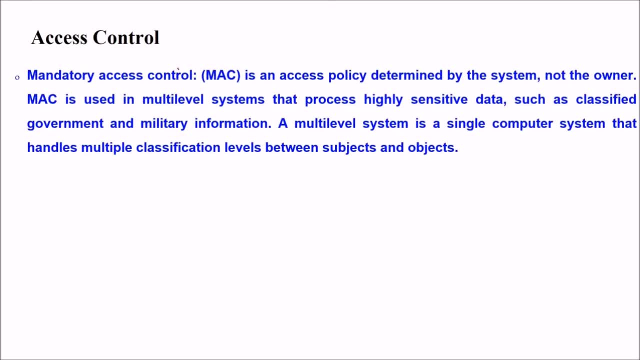 control over its access policy. like the owner, Then MAC, Mandatory Access Control. MAC is access policy determined by the system, not the owner. so msa is used in multi-level system that process highly sensitive data such as classified government and military information, so multi-level. 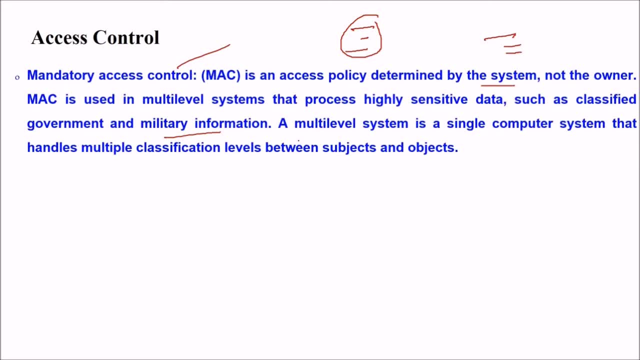 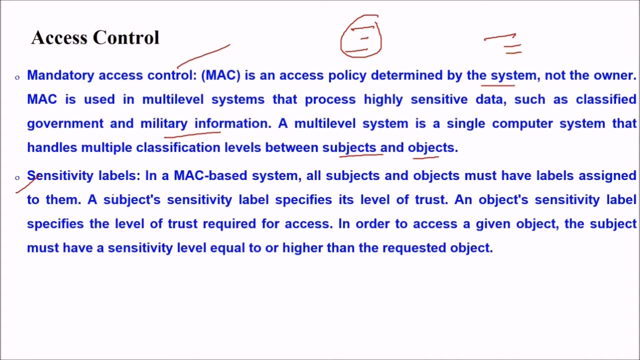 multi-level system is a single computer system that has multiple classification level subjects and objects. they are just not only one, they are multi-level subjects and objects so they can have sensitivity levels. in mandatory access control systems all subjects and objects must have a label associated with them, assigned to them. so subject sensitivity label provides its level of. 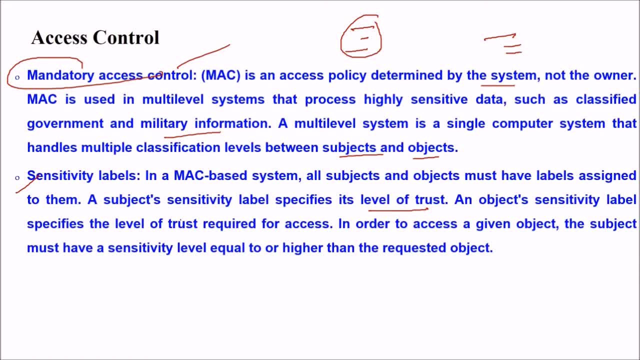 trust. first of all, an object sensitivity label. it specifies the level of trust required for the access. so in order to gain the access to a given object, subject must have a sensitivity level which is either equal to or higher than the requested object. what about data import? and 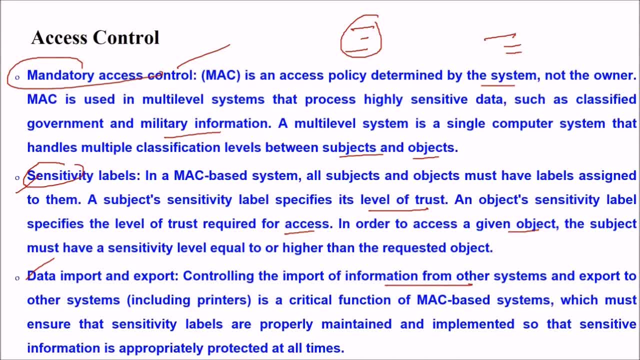 export, controlling the import of information from other system, that is, from other system, or exporting to other system, which include the printers. also, it's a critical function of making a mac based system. that is, mandatory access control, which must ensure the sensitivity labels are properly maintained and implemented so that the sensitive information is always protected all the times. 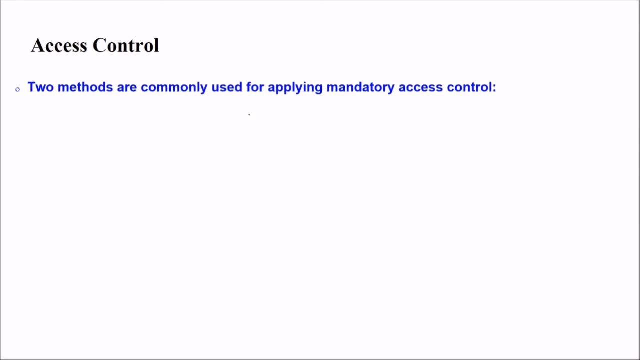 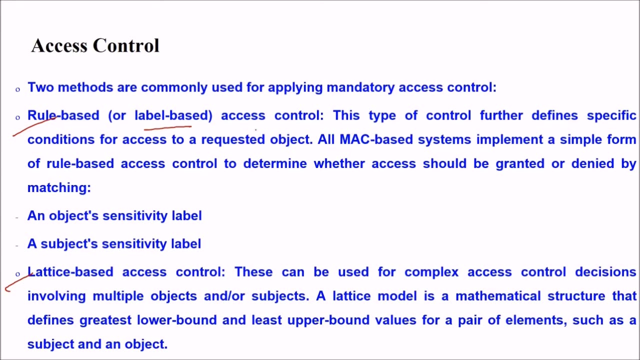 appropriately. there are two methods which are commonly used for applying this mac. first is rule based, the second is lattice based control. access control in rule based or label based access control, the. the control further defines specific conditions for access to the request requested object. all mac based system implement a simple form of rule based access control to determine whether access 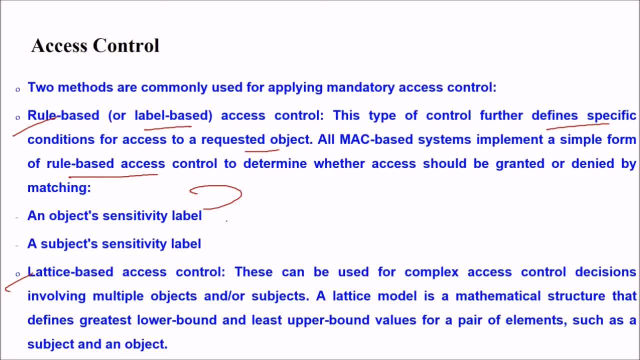 should be granted or denied by matching first, then first an object sensitivity label, then the subject sensitivity level. and what about the second method for applying mac, that is, the lattice based control, access control? this can be used for complex access control decision which involve the multiple objects and subjects. so a lattice model is a mathematical structure so that defines a greatest lower bound. 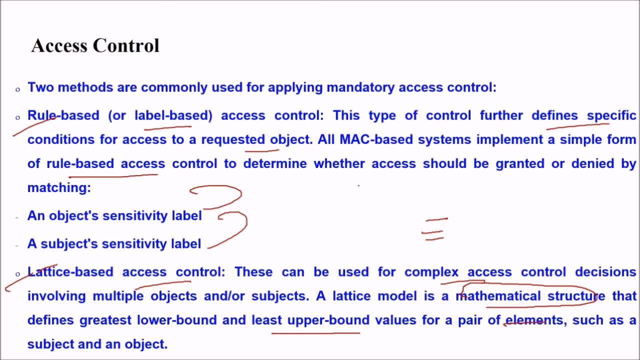 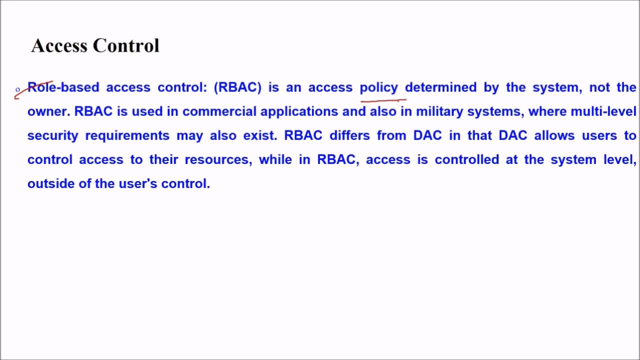 and the least upper bound values of for a pair of element for, such as for subject and object. then we have rbse, that is, role based access control. so this is access policy determined by the system, not the owner. again, not the owner, but by the system. so role based access control is used in commercial. 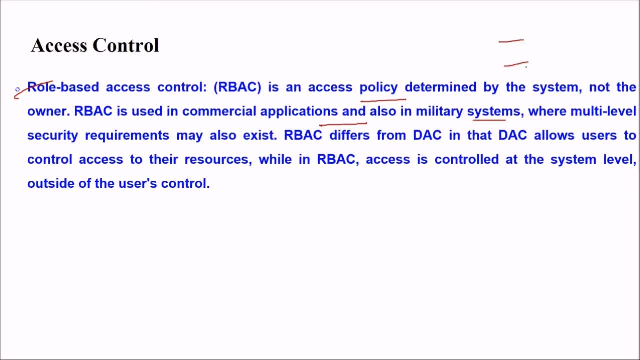 application and also military systems where we have multi level security requirements. this may also exist. so rbse differ from dac. how in this, dac allow user to control access to their resources, while rbse access is controlled at the system level, outside the scope of the user control. 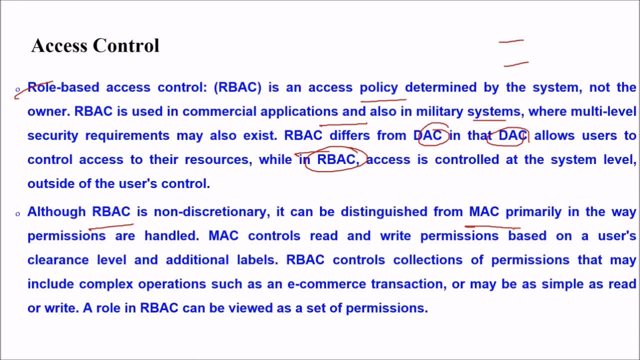 though this rbse is non-discretionary, it can be distinguished from mac primarily in the way the permissions are handled, because mac controls read and write permission based on the user clearance level and additional levels, and rbse control collections of permission that may include complex operation also, such as e-commerce transaction, or maybe you know simple as read, or 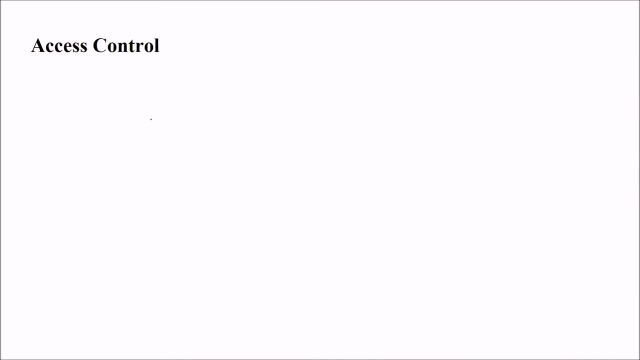 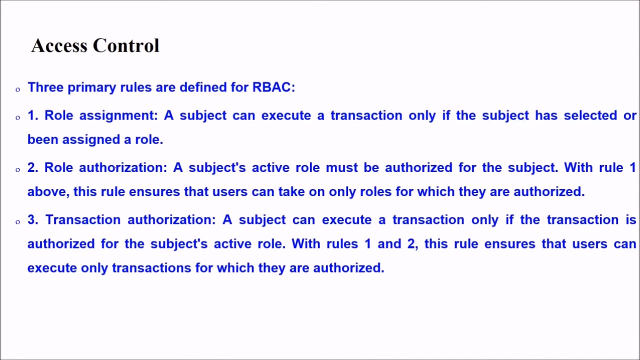 write. so role of rbse can be viewed as a set of permissions. so there are three primary rules that are defined for rbse. first is your role assignment, role authorization and then transaction authorization. so role assignment in rbse are the set of permissions that are usually used for the service. then it is also used to handle the role of rbse. 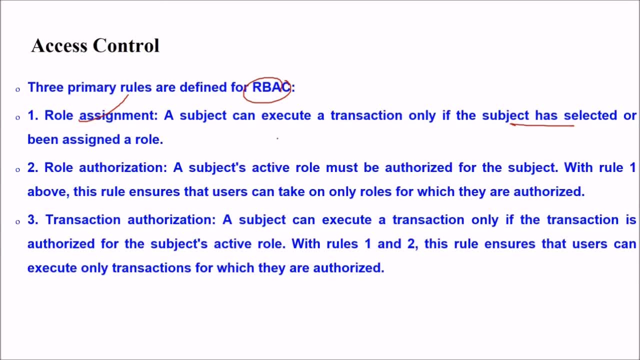 subject can execute a transaction only if the subject has selected or been assigned a role. What about role authorization? A subject's active role must be authorized for the subject. So with rule 1, these rules ensure that the user can take only roles for which they are actually. 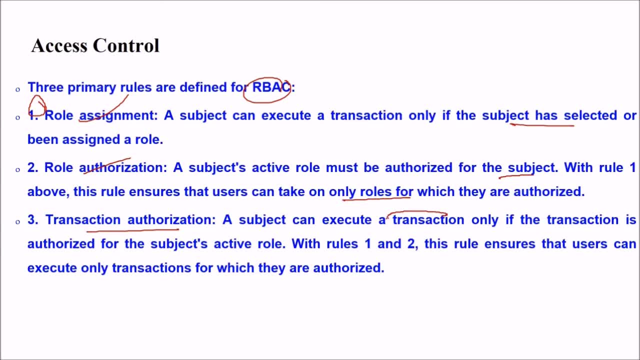 authorized. What about transaction authorization? A subject can execute transaction only if the transaction is authorized for the subject's active role. And with these two rules? this rule ensures that the users can execute only transactions for which they are actually authorized, So additional constraint may be applied as well. You know the rules can be. 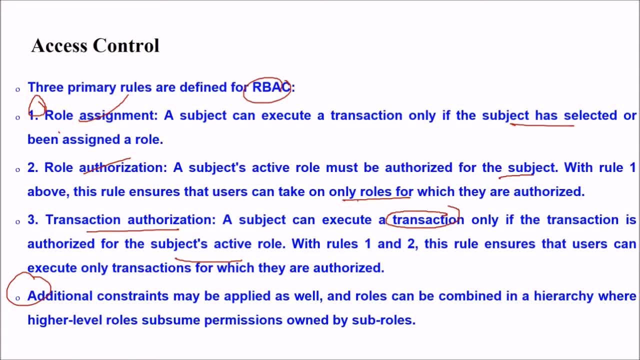 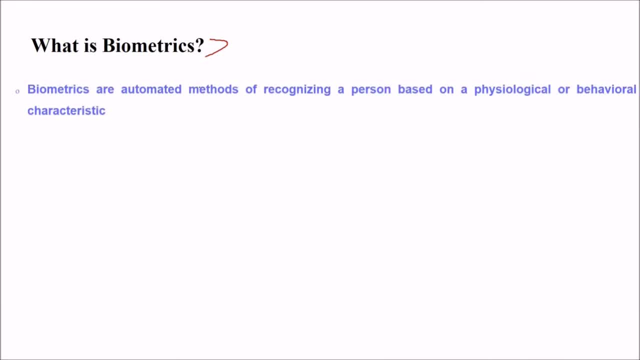 combined in a hierarchy where higher-level roles subsumes the permission owned by the sub-roles. So most IT vendors offer this RBSE in one of the four more products. Now we come to the biometrics. What is biometrics in access control Biometrics? they are automated methods of recognizing a. 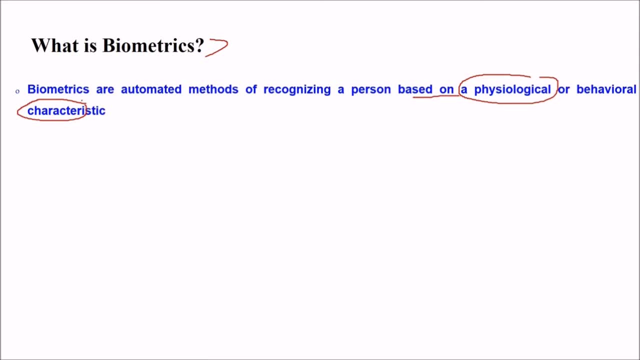 person, which is based on the physiological and behavioral characteristics- Again, physiological and behavioral characteristics. So these features are measured in this. Biometrics are face, fingerprint, hand geometry, handwriting, iris, retina, vein and vein and voice. So identification, person certification. 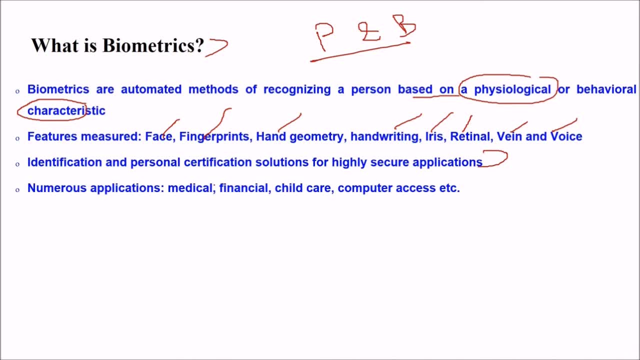 solution for high risk, secure application. you need it, So there are numerous applications. It may be medical, financial, child care, computer access, And biometrics actually has replaced traditional authentication and it provides better security. Convenient also And accountability is also there. Applications on fraud detection, fraud tolerance, deterrence. 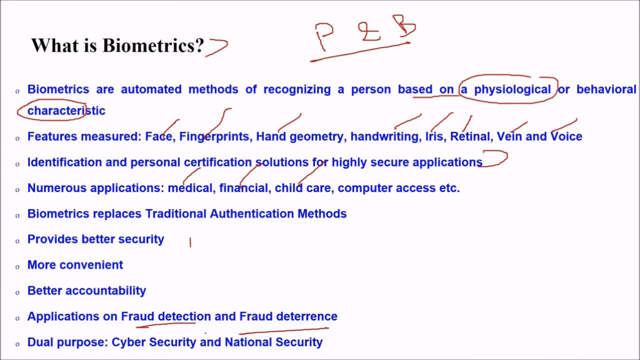 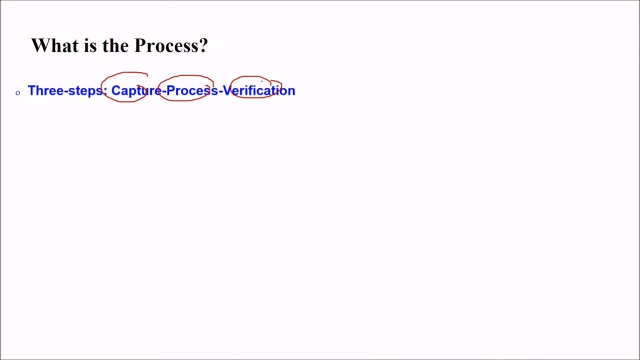 is biometrics. It solves dual purpose: First your cybersecurity and then national security also. So what is the process? There are three step process. First is capturing, processing and verification. Capture process: verification: Biometrics involve three process: Capture: 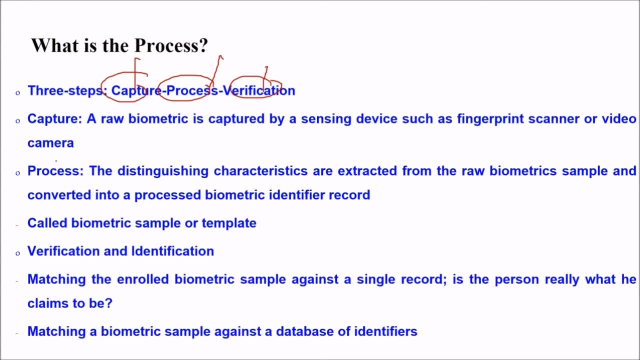 process and verification. What about capturing, then processing and then verification and validation? In capturing, a raw biometric is captured by the sensing device such as fingerprint scanner or video camera. Now the distinguished characteristics are extracted from the raw. 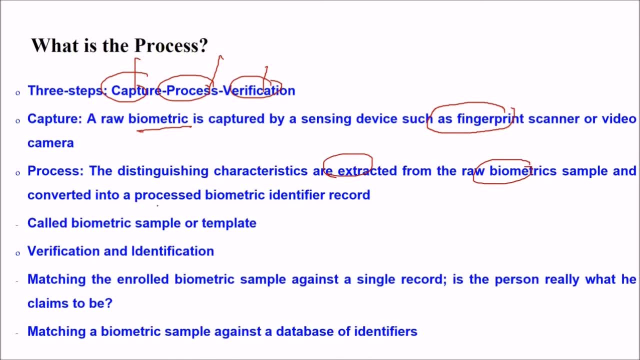 biometric sample which is taken, just now taken, and they convert it into process biometric identifier record. We also call this is called biometric sample or template. Now we also call this is called biometric sample or template. Now, we also call this is called biometric sample or template. 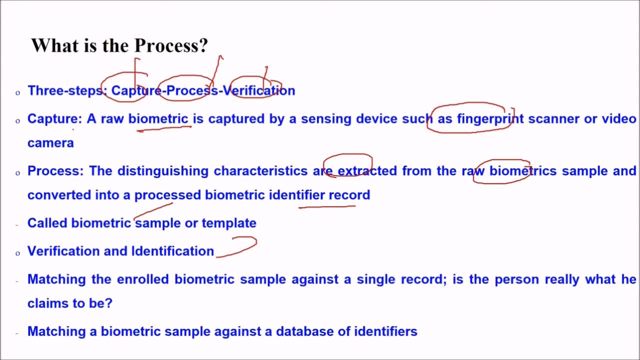 What about verification and identification? Now, we have captured and now processed also, So we have records with us. So matching the enrolled biometric sample against the single record. So this is the person, really what he claims to be. So matching a biometric sample against the database. 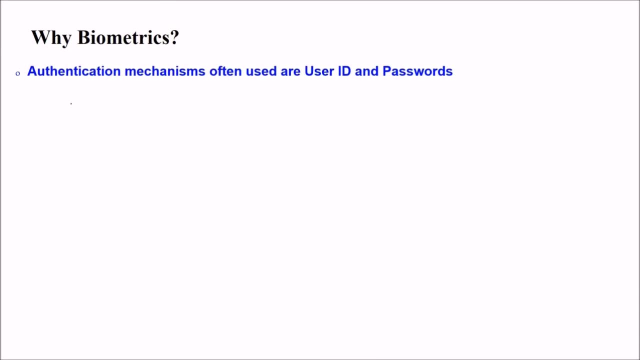 of identifier is the verification and the validation, So authentication mechanism. they often use the IDs and password, So password mechanisms have vulnerability. You can steal password always. So biometric systems are less prone to attacks. Why? Because we need. 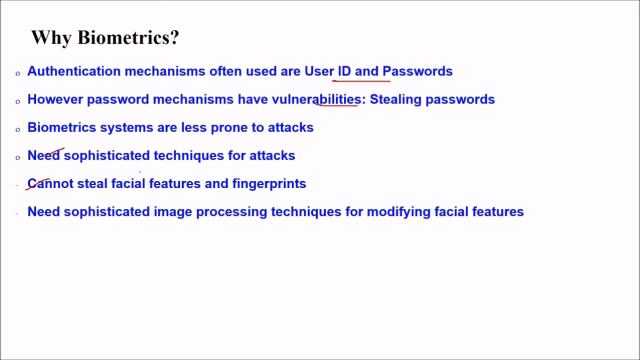 sophisticated techniques for attacks. You cannot steal facial features or fingers. you know This is impractical. So it needs sophisticated image processing technique for modifying the facial features also. So biometric systems are quite convenient and you need not to have multiple. 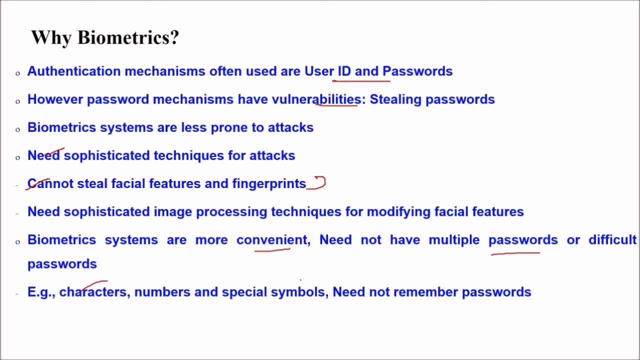 passwords or difficult passwords, For example, characters, numbers, special symbols and you know we may not remember. also, You don't have to carry the cards and tokens. Contability also is good, Why You can determine who accesses the system with minimum complex. 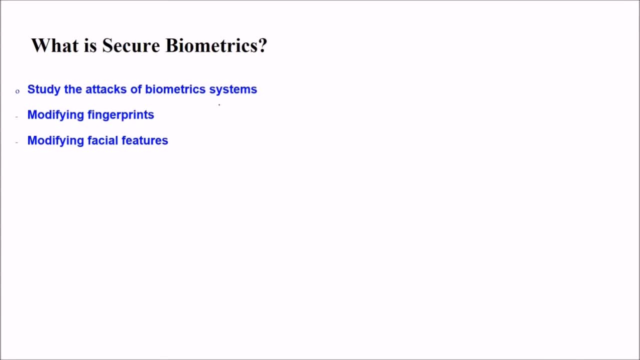 city. So what is secure? biometrics: We study the attacks of biometric systems. That is, you can modify the fingerprints, you can modify the facial features and we can develop a security policy and model for the system. That is the application, which are independent and application specific. 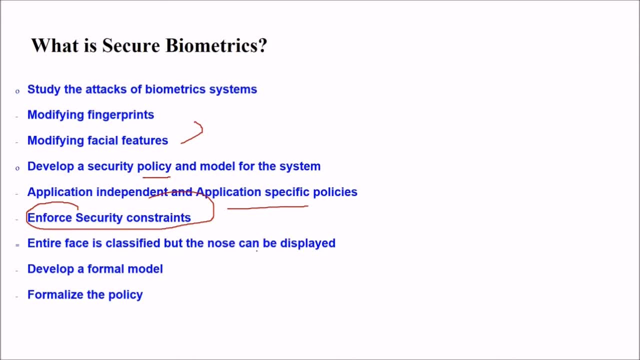 policies. We can enforce the security constraints- Entire face is classified, but the nose can be displayed- Develop a formal web model or formalize the policy So we can also design the system and identify security critical components, like even reference monitor for biometric systems. 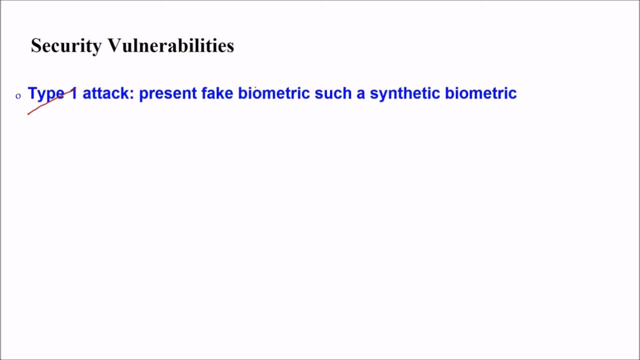 There are certain security vulnerabilities. First is type 1 attack: Person can fake biometrics such as synthetic biometrics. Type 2 attack: submit a previously intercepted biometric data and you can replay it. Type 3 attack, compromising the feature extractor module to give results designed by the attacker. 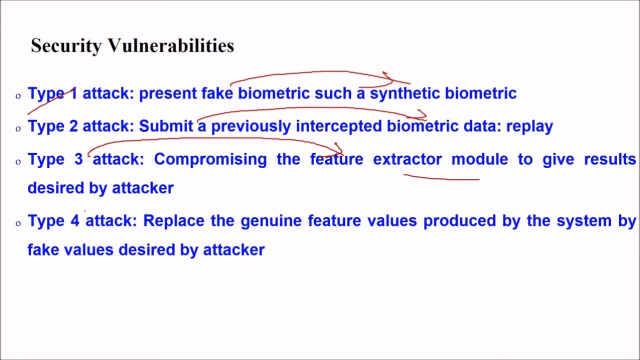 That is what image processing has been done. It can be manipulated And type 4, replace the genuine feature values produced by the system by the fake values designed by the attacker. And type 5 attack produce a high number of matching results. Type 6 attack attack the template database itself. Go to: 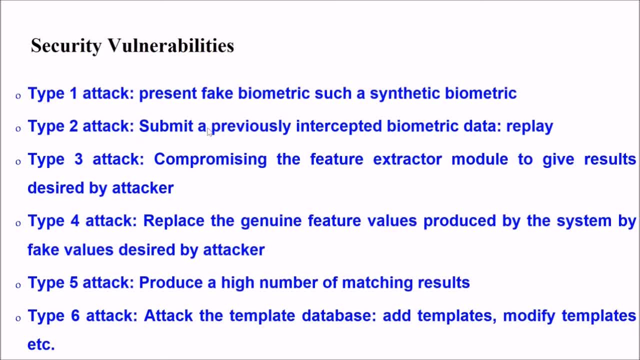 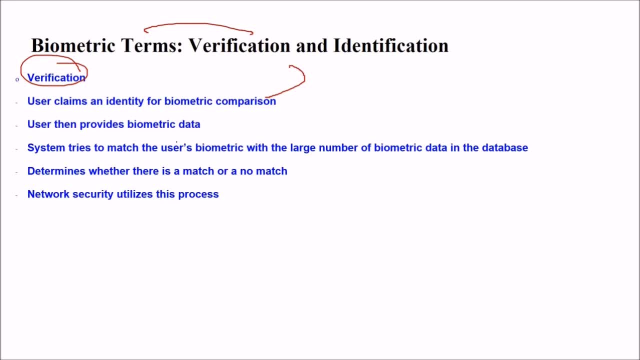 go to the database, Add a template, modify the template. This is the type six attack. So, in terms of biometric verification, identification verification- user claims an identity for biometric comparison. This provider provides biometric data. The system tries to match the user's biometric. 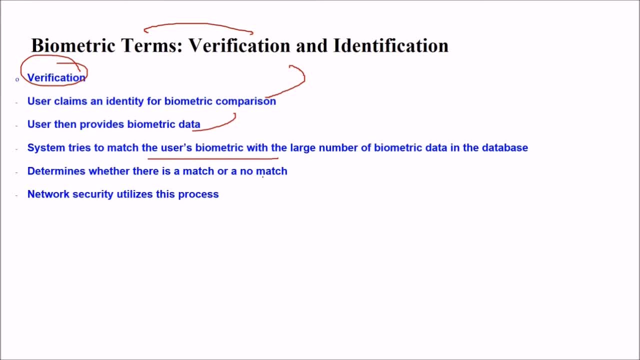 which has given a large amount of biometric data in the database and it determines whether there is a match or a mismatch. Network security utilizes this process. What about identification in the biometric terms? user has no claim on identity. He doesn't claim identity, but he gives. 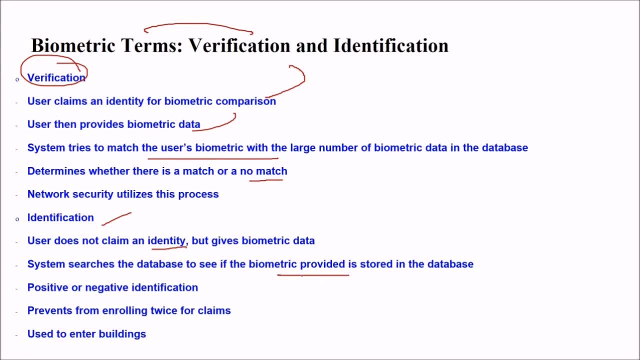 biometric data System searches the database to see if the biometric provided is stored in the database. We can have a positive or negative identification and this actually prevents from enrolling the twice for games and use for entering buildings etc. So biometric process. 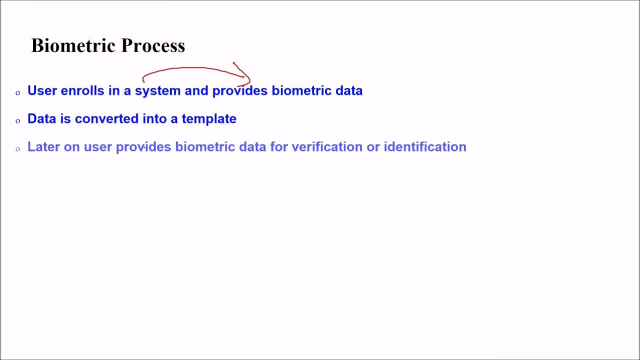 user enrolls in a system and provide the biometric data. Data is converted to a template. Later, the user provides the biometric data for verification and validation. The latter biometric data is converted into a template. The verification identification template is compared with. 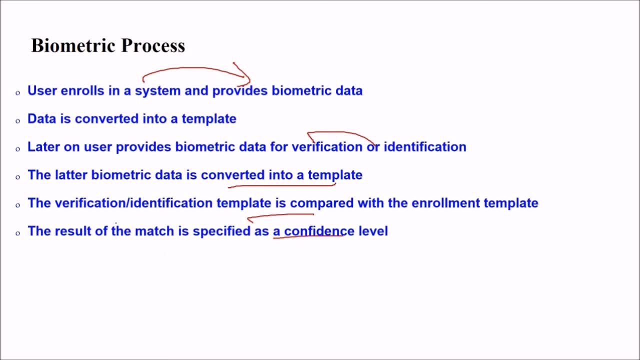 an enrollment template and the result of the match is specified as a confidence level. So this confidence level is compared to the threshold level and if the confidence level actually exceeds the threshold we say there is a match. If not, there is no match. 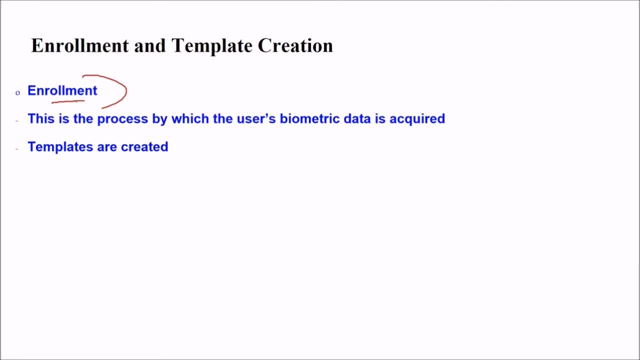 What about the enrollment and template creation? In enrollment, there is a process. This is actually a process by which the user's biometric data is acquired, Templates are created. And about presentation? users present biometric data using the hardware such as scanning. 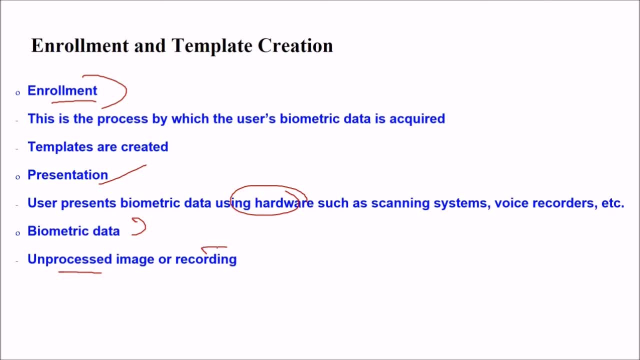 systems or voice recorder etc. And biometric data. they can be unprocessed image or, say, recording And feature extraction. now this image processing comes: We locate and encode the distinctive characteristics from the biometric data, The data types and associated biometric technologies. 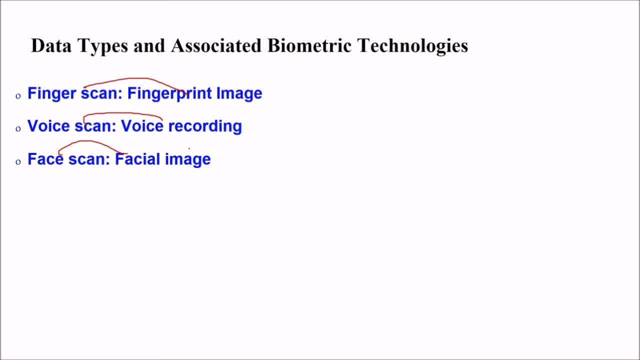 we have finger scan, fingerprint image, voice scan, voice recording, face scan- that is face image. your facial image. iris- that is iris image, retina, retina image, hand scan. image of complete hand signature. image of the signature and the key stroke. 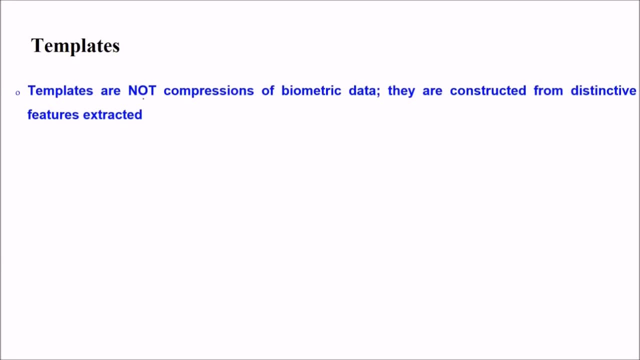 scan, that is, recording, the recording of the character types. So what are the templates? These templates are not compression of biometric data, They are the. they are constructed from the distinctive features which has been extracted. You cannot reconstruct the biometric. 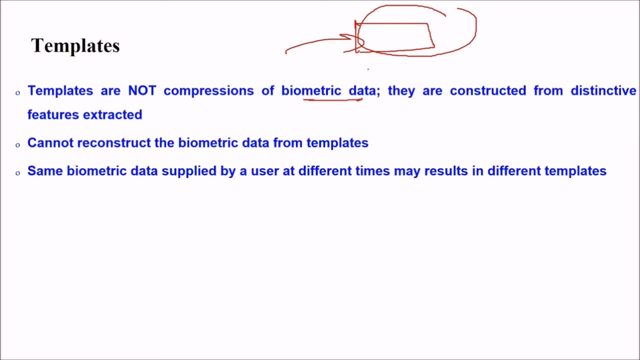 data from the templates. So some same biometric data supplied by the user at different times may result in different templates also. So when the biometric algorithm is applied to these templates, it will recognize them as the same biometric data. And templates may consist of strings of. 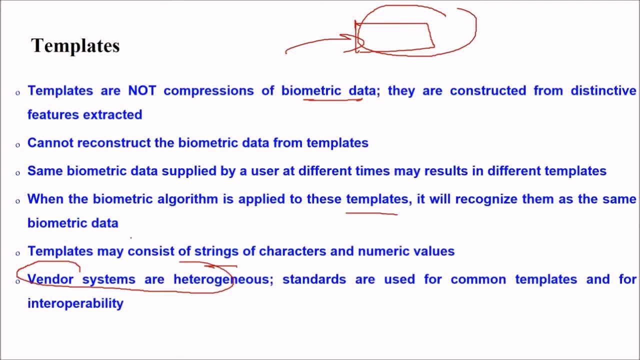 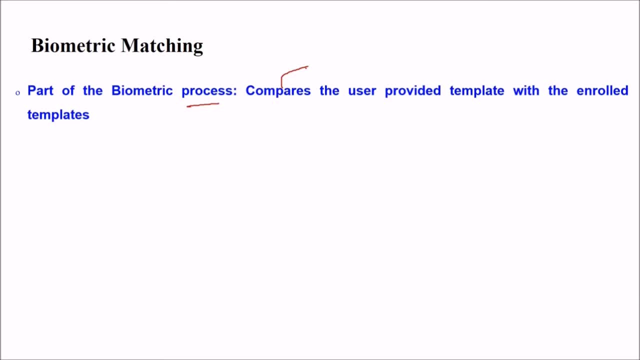 characters or say numeric values, And the vendor systems are heterogeneous. So the standards are used for common templates and for interoperability also. So in biometric matching- part of the biometric process- it compares the user provided template with the enrolled templates. 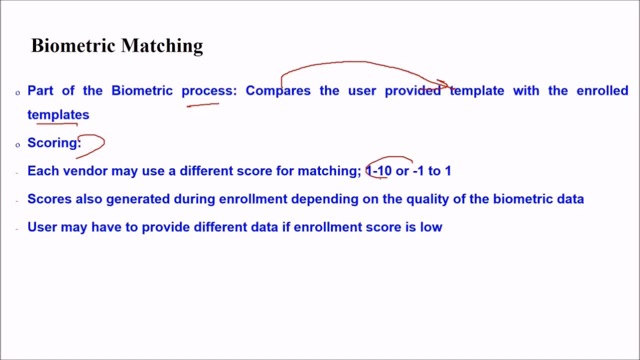 So scoring. So each vendor may use a different score for matching 1 to 10 or minus 1 to These scores. they are also generated during the enrolment, depending on the quality of the biometric data, And the user may have to provide different data if the enrolment score is low. 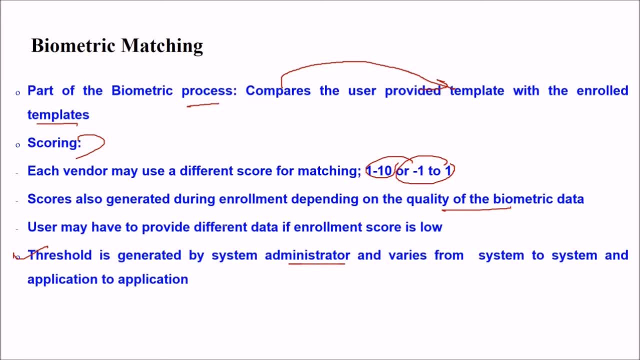 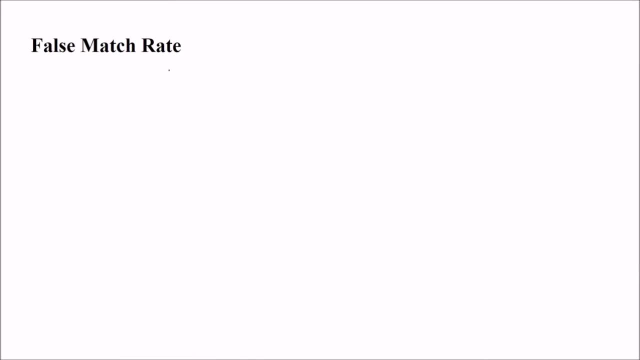 And the threshold is generated by a system administrator and it varies from system to system and application to application And decision depending on a match. 100% is generally not possible. What is the false match rate System gives a false positive by matching a user biometric with another user's enrolment. 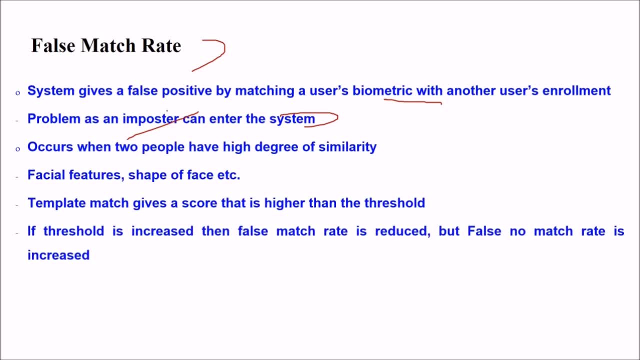 So problem as an imposter can enter the system. this is a problem, So it occurs when two people have high degree of similarity. They may have same facial features. shape of face are equal, So template matches gives a score that is higher than the threshold. 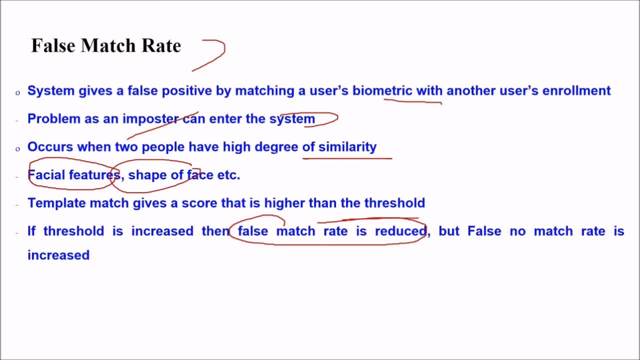 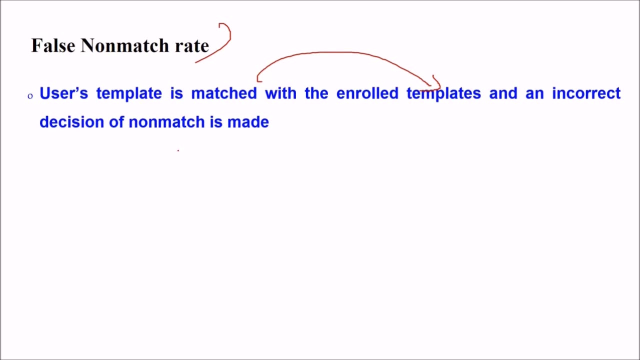 If threshold is increased, then the false match is reduced But the false no match rate is increased. So false match rate may be used to eliminate the non-matches and then to do the further matching. This false non-match rate. user's template is matched with the enrolled template and an incorrect decision is non-match is made. 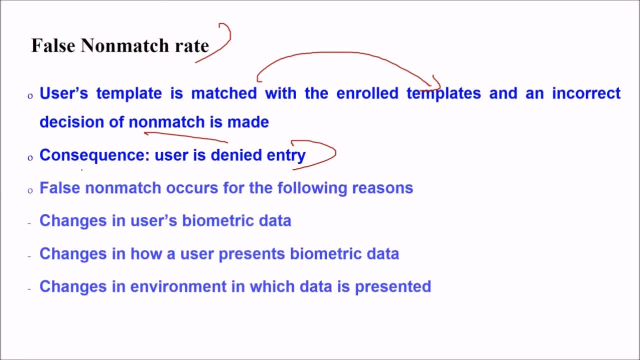 So the concept is. the result is the user is denied the entry And false non-match occur for the reasons like changes in the user's biometric data, changes in how a user present biometric data and changes in the environment in which the data is present. 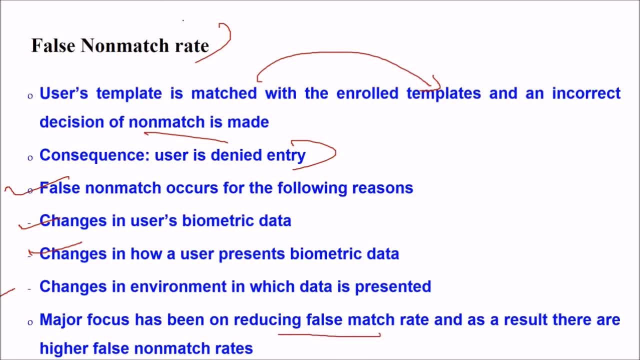 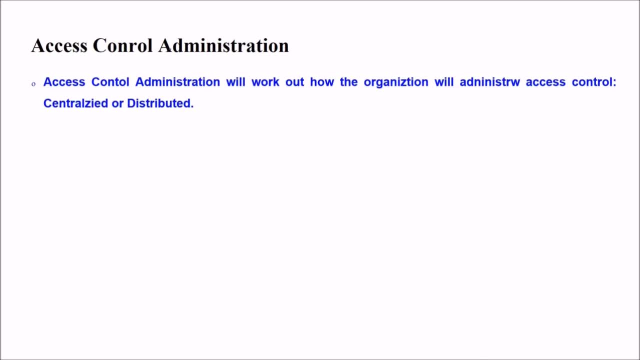 So the major focus is on reducing the false match rate and, as a result, there are higher false non-match rates. Access control administration: See this. access control administration will work out how the organization will administer access control. It may be centralized. it may be distributed. 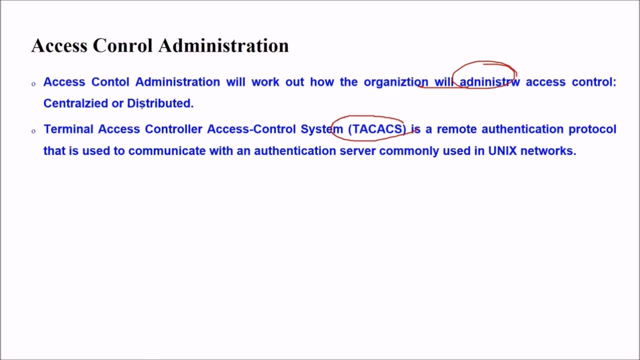 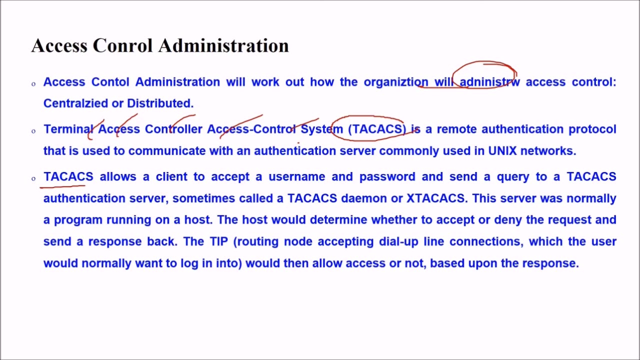 So this TACACS terminal access control system is a remote authentication protocol Terminal access controller, access control system which is used to communicate with authentication server commonly used in Unix. This TACACS allows client to accept the user and password and it sends a query to TACACS authentication server. 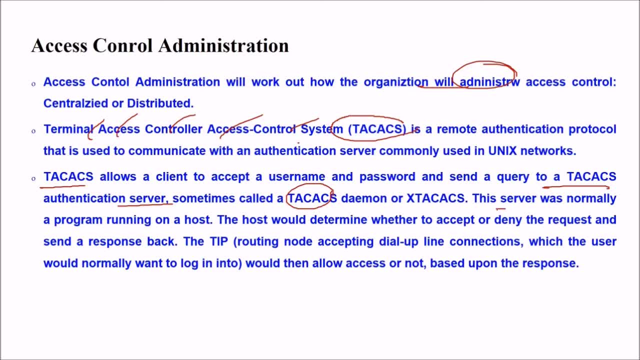 Sometimes called as TACACS daemon or X-TACACS. So this server was normally a program running on a host, So host would determine whether to accept or deny the request or it will send a response back, The TIP, that is the routing name node accepting dial-up line connections that the user would normally want to login into. 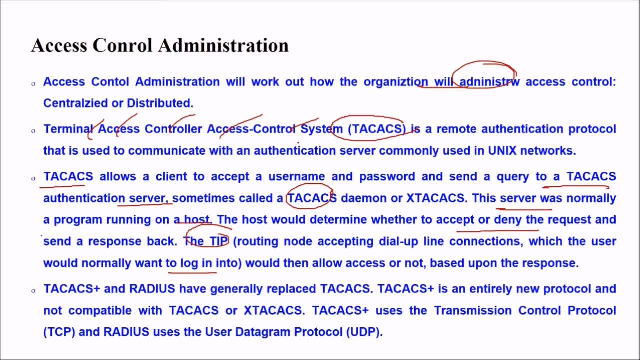 would then allow access or not, based on the response. So TACACS plus RADIUS, they have generally replaced the TACACS. This plus is an entirely new protocol and is not compatible with the earlier one or this X-TACACS. This plus uses the transmission control protocol TCP. 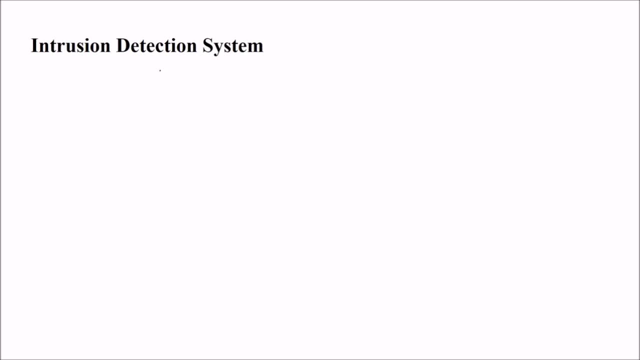 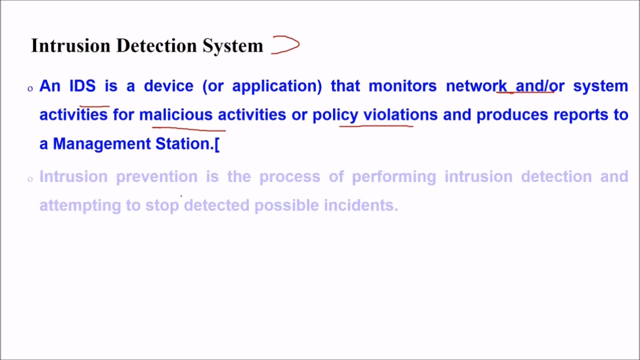 And RADIUS uses the UDP user data protocol. What about the intrusion detection system, IDS? This is a device or application that monitors network or system activities for certain malicious activities or certain violation in the policies And we produce reports to the management section. Intrusion prevents or prevention is the process of performing intrusion detection and attempting to stop detected possible incidents. 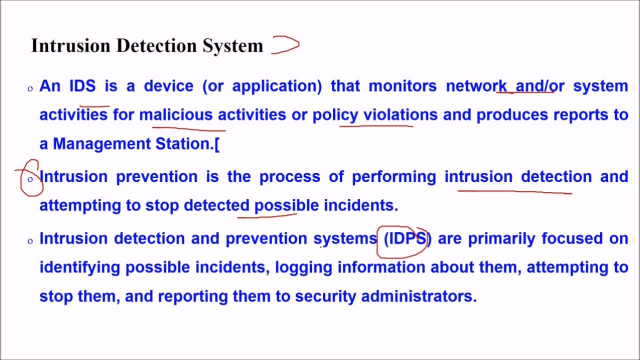 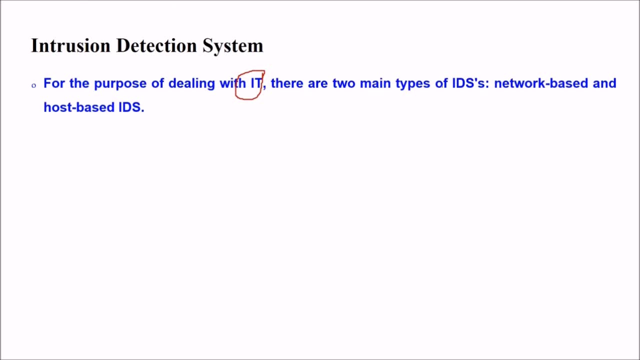 So this IDPS or intrusion detection and prevention system. They are primarily focused on identifying possible incidents, log information about them, attempting to stop them and reporting them to the administrator to take necessary action And the purpose of dealing with this intrusion. There are two types of IDS: network based and host based intrusion detection system.